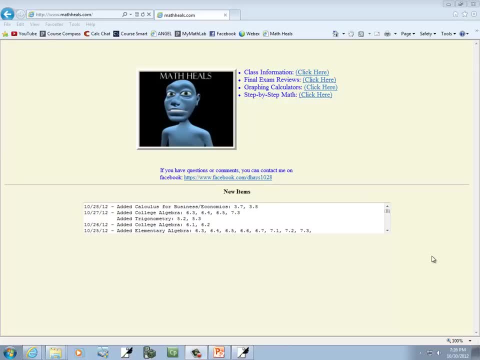 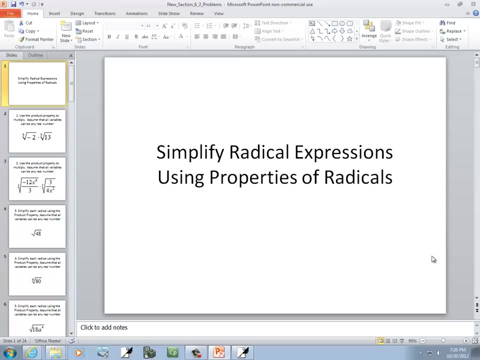 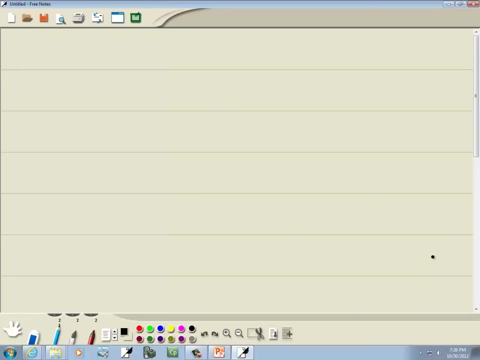 This is mathhealscom, where you can go to find more links to math YouTube videos. Let's take a look at simplifying radical expressions using properties of radicals, And the first thing we're going to talk about is the product property, And we'll have various properties. 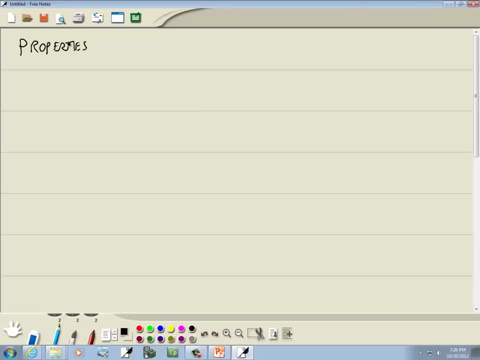 Now this one. there's different versions of this, different ways you can write it, But basically, if you're Yeah, B is probably okay, but let me choose different. I'll put P there. If you're multiplying two radicals together and the indexes are the same, the number in this slot right here. 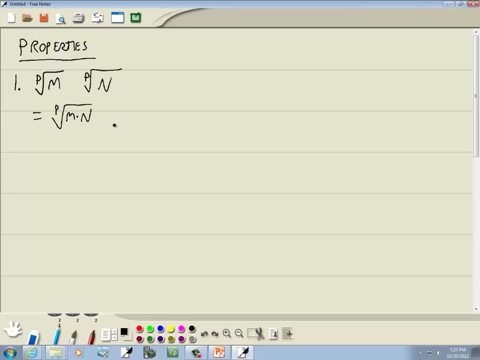 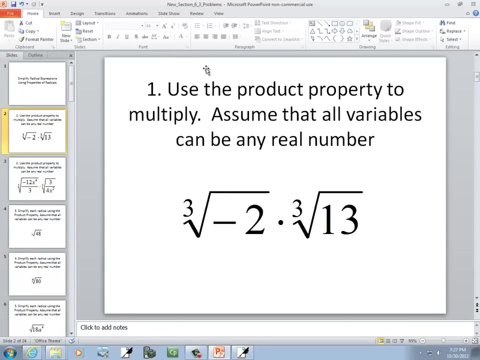 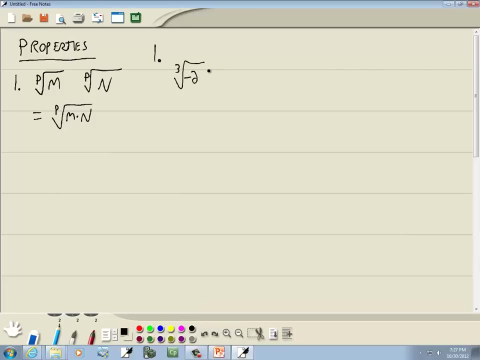 then you can put them underneath a single radical. like that, You can also go the other direction. If you have this, you can split it into two separate radicals. Excuse me So this first problem. here We have the cube root of negative 2 times the cube root of 13.. 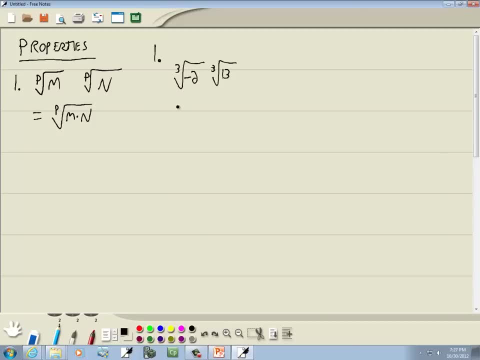 It says: use the product property to multiply. assume all variables can be any real numbers. Since the indexes are the same, we can multiply these together and put them underneath a single radical. So I've got negative 2 times 13. Which gives us a negative 26.. 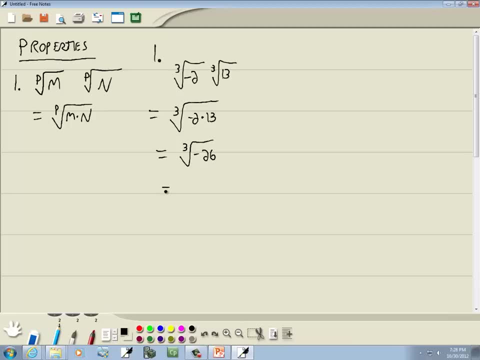 Now remember: whenever you have a negative inside of a radical with an odd index, you can take that negative and bring it on the outside. So this gives us negative cube root of 26.. Let's take a look at our next one. 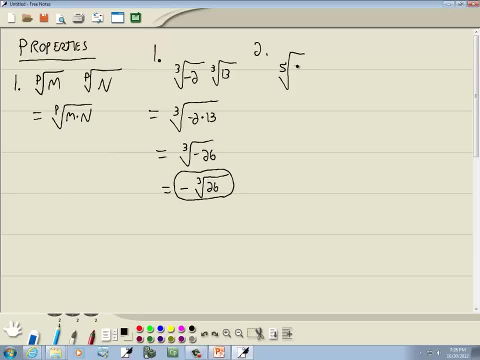 We've got the fifth root of negative 12x to the fourth Over 3 times the fifth root of 3 over 4x squared. Now we're multiplying these together, so I'll put them underneath a single radical with the fifth root. 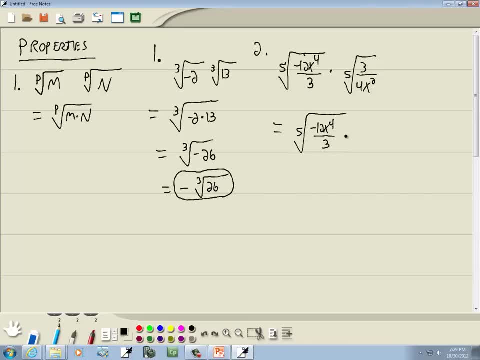 So I've got negative 12x to the fourth, over 3 times 3 over 4x squared. Now we can do something else. Some simplifying here. These three is going to cancel, And let me write it down again before I do any more simplifying. 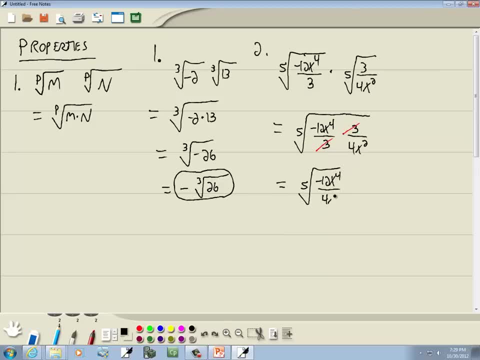 And I've got negative 12x to the fourth over 4x squared. Well, we've got negative 12 here, We've got 4 here. The both is by 4.. 4 divided by 4 is 1.. 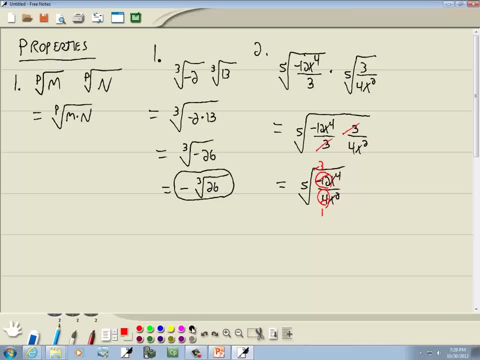 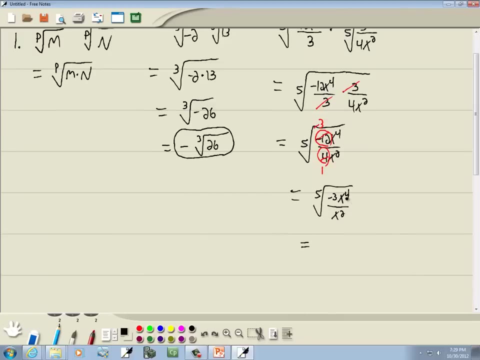 Negative 12 divided by 4 is negative 3.. So we've got the fifth root of negative 3.. 3x to the fourth over x squared. Now remember: if you have x to a power, over x to a power, you subtract a smaller exponent from a larger one. 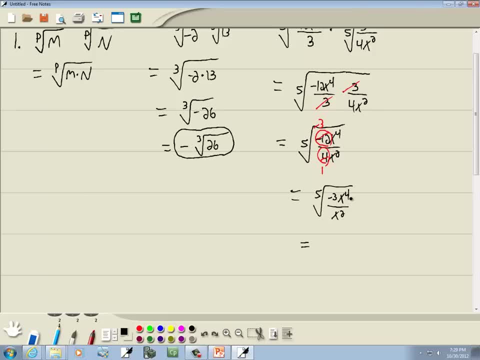 4 minus 2 gives us 2.. And we put x to that power where the larger one was, which was on top. When I say larger, I'm talking about the exponent. So we've got negative 3x squared over 1.. 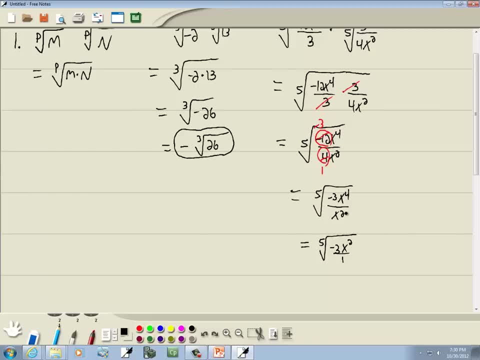 So again, subtract a smaller exponent from a larger one: 4 minus 2 is 2. And we have x to that power where the larger exponent was, which was on top, Which gives us the fifth root of negative 3x squared. 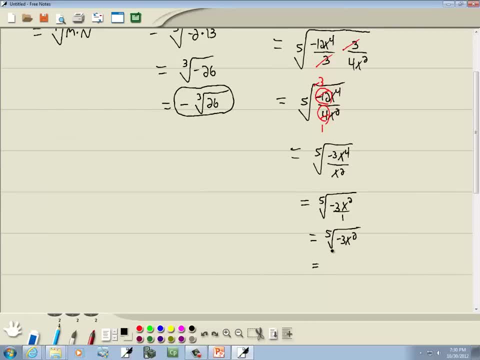 Now remember, whenever our index is odd and we have a negative number inside, we can take that negative and put it on the outside of the radical. So we've got negative fifth root of 3x squared And that's our answer. 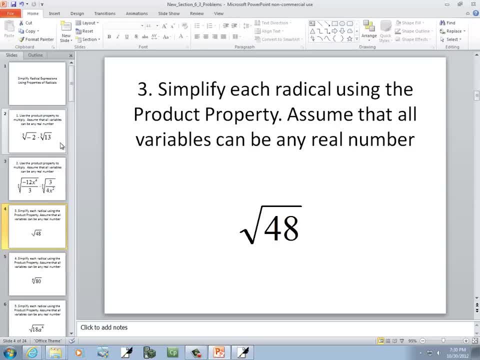 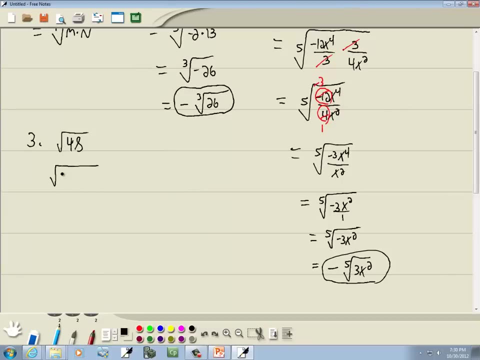 Now this next one. It's a little bit different. Remember how I said: there's different ways you can work the product property. It says: simplify each radical using the product property. So all variables can be in real numbers. Well, 48 is 2 times 2 times 2.. 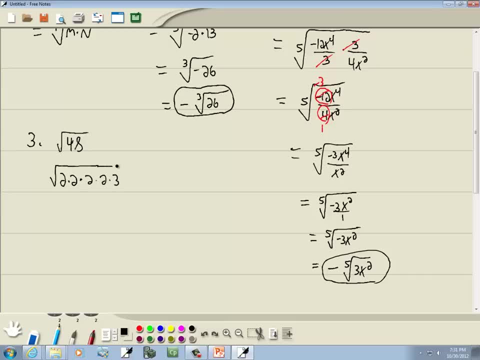 2, 4, 8, 16, 48.. So 2, 4, 8,, 16,, 48.. Okay Now, our index is 2.. There is no number in this little slot right here. 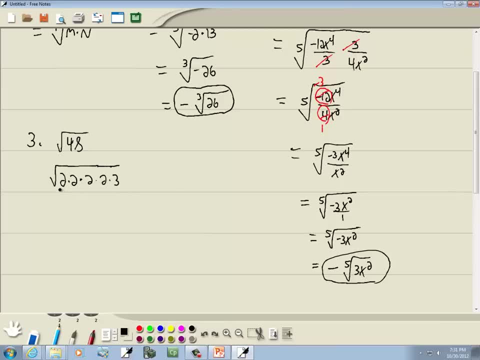 So it's, by default, 2 square root, which means we're looking for pairs of something. Here's a pair of 2s and here's a pair of 2s, So a pair of 2s is going to come out. 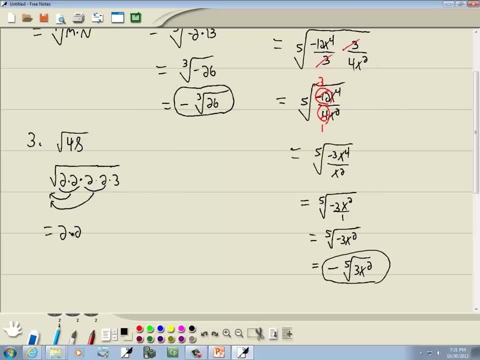 And this pair of 2s is going to come out Now. when they come out, they come out with multiplication in between them, So it's 2 times 2.. And then we've got a 3 inside. 2 times 2 is 4.. 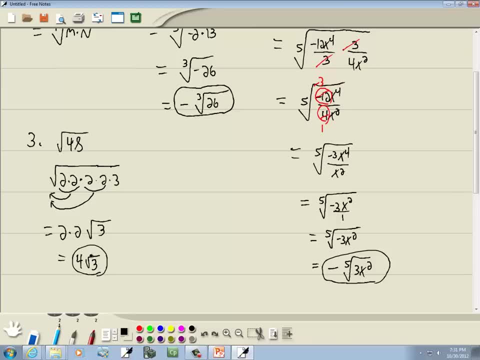 So our answer is 4 square root of 3.. Now, well, why is this the product property? Well, I could split this up. I could split this up as the square root of 4 times square root of 4 times square root of 3.. 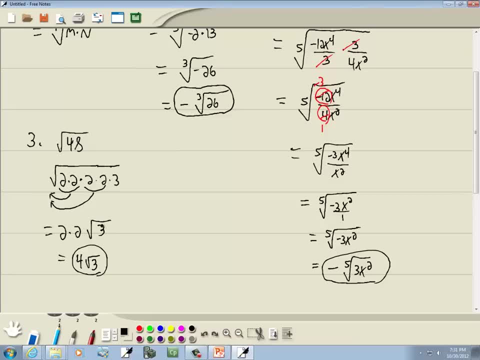 And then square root of 4 is 2.. Square root of 4 is 2.. And then the square root of 3.. We never show those steps, But that's implied when we're doing this. Okay, Let's look at the fourth root of 80.. 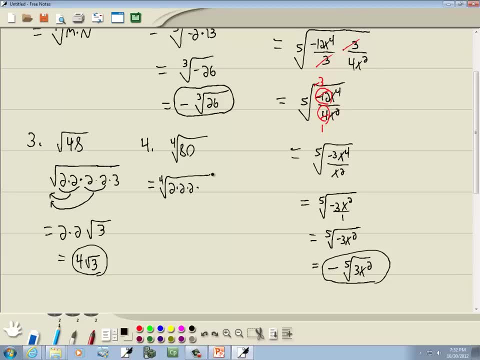 80. That's 2, 4,, 8,, 16,, 48. Um times 10. So 2 times 5.. 2, 4, 8, 16.. Okay, That'd be right. 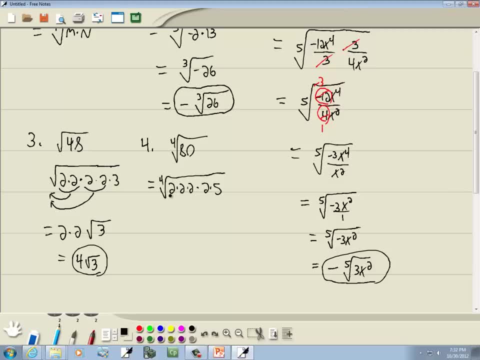 Uh, now our index is 4.. Which means we're looking for a set of 4 of something. Well, here's 4 2s. So those 4 2s are going to come out in front as a single 2.. 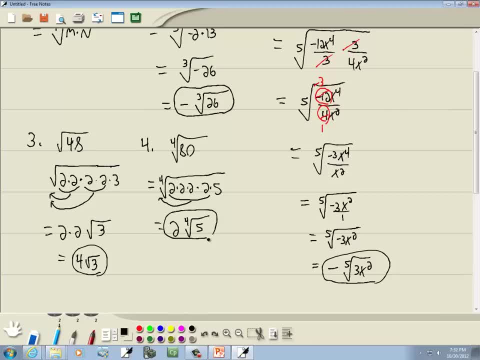 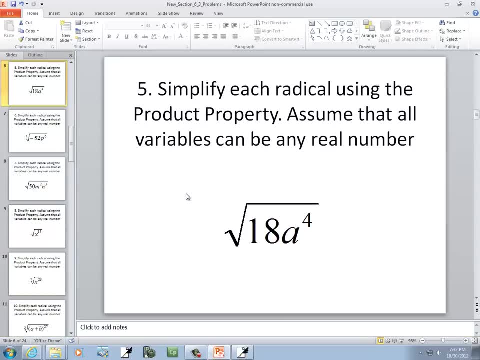 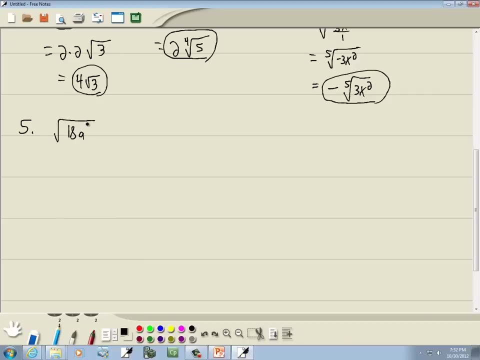 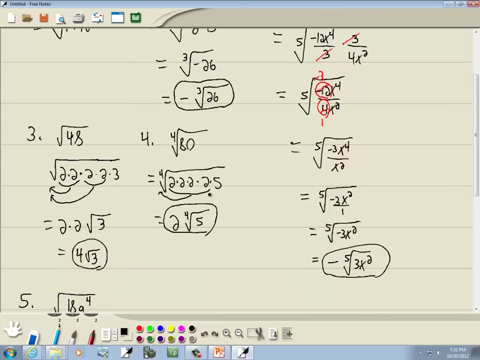 So we've got 2, 4th root of 5. And that's our answer Here. we've got square root of 18a to the 4th. Now, um, up to now, these examples, um, nothing's come out of the radical there, except for a negative. 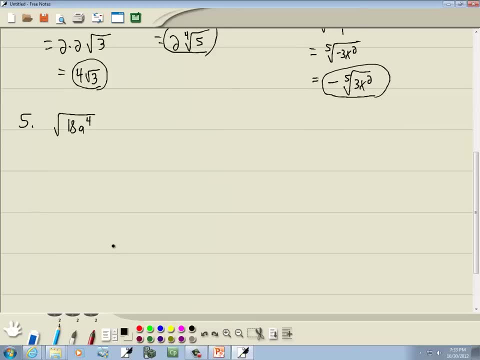 Nothing here but a negative. Here's a 2.. Here's a 4. This one: we're going to bring something, something out, And we'll talk more about that. Um 18 is 2 times 3 times 3.. 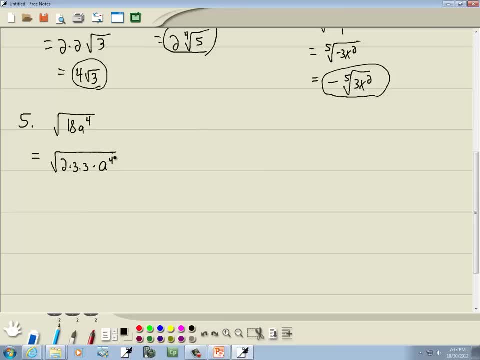 Now a to the 4th. We'll come back to that. First let's look at the numbers. Here's a pair of 3s, So those are going to come out as a single 3.. Okay, And now the a's. 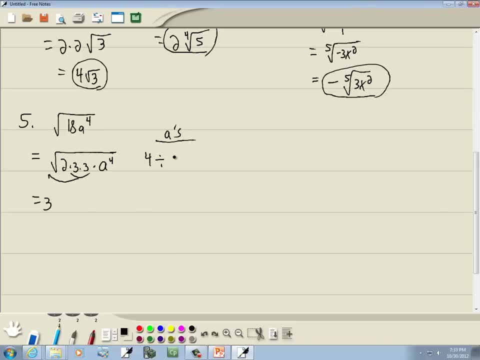 What you do is you take your power, which is 4.. You divide by your index. Index is this number in a slot, And if it's a square root, it's by d4.. So you're going to have a default 2.. 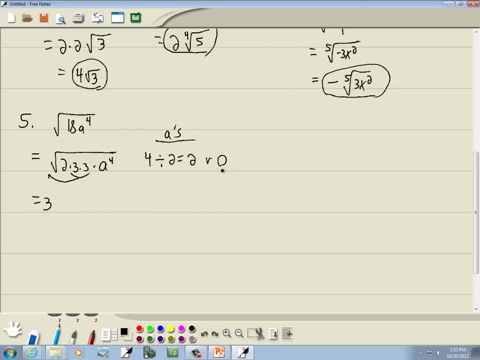 So 4 divided by 2 is 2, with a remainder of 0. This is old style division. Now, this first part here tells us how many a's come out, And this tells us how many a's stay in. So that tells us we're going to have 2 a's come out. 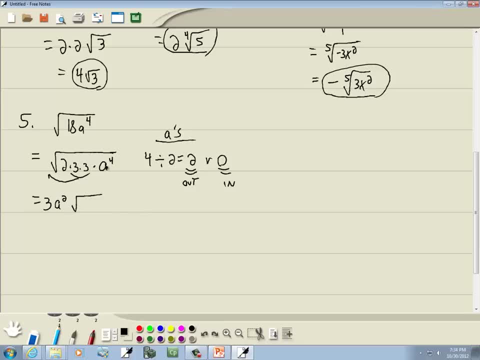 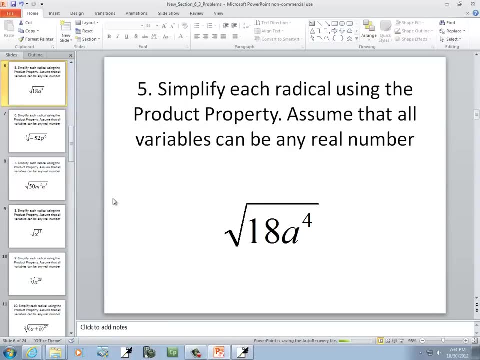 And 0 a's stay inside. Well, the 3s are gone, The a's are all gone, So we've got just a 2 in here Now. um, it says: Uh, Assume that all variables can be any real number. 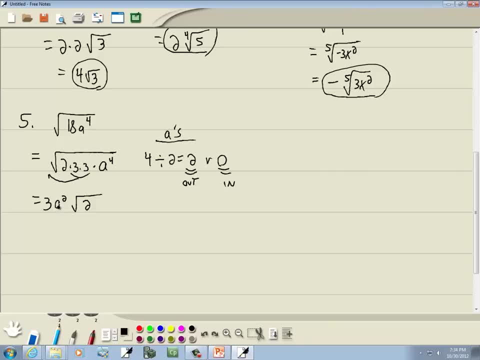 That means that we- um, this can be positive, it can be negative. Well, you can never have a negative number come out of a square root or any radical with an even index. Now, odd index is fine, Like up here. we had a negative number come out, which is fine. 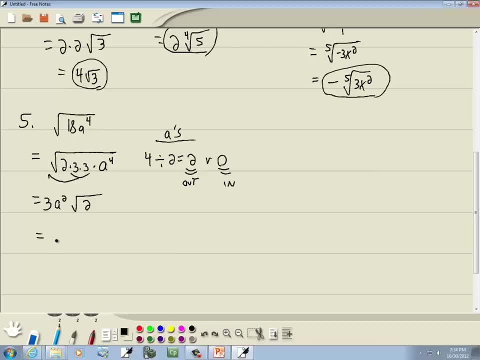 But when your index is even, you can't have a negative number come out. Well, how we ensure that it's positive is: whatever variable comes out. you put absolute value bars around it, Like that Now, in this particular case, um the a squared. well, when you square something, it's always. 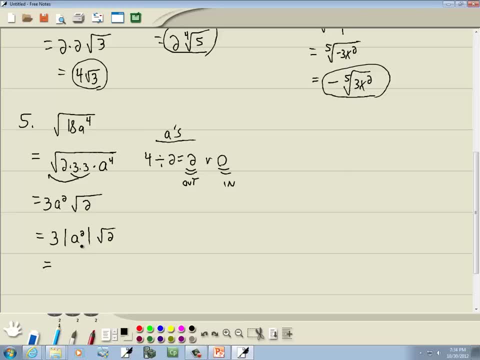 positive, isn't it Negative? 2 squared is positive 4, 2 squared is positive 4.. So those absolute value bars aren't necessary here. So we've got 3 a squared square root of 2.. But again, any time your index is even and you're bringing out a variable, you have to. 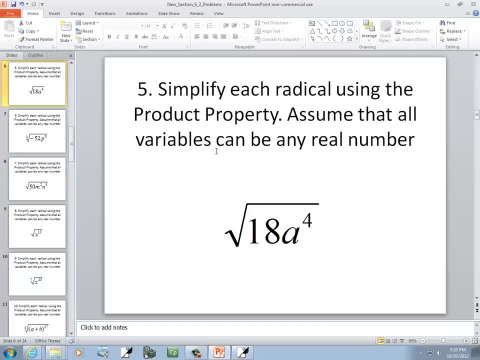 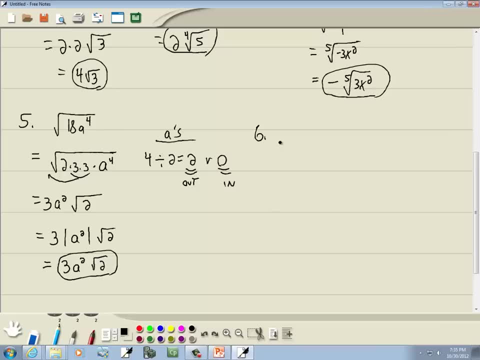 think of the absolute value bars. Let's look at, uh, number 6.. We've got the cube root of negative 52 p to the 6.. Okay, let's look at the number. Well, first off, we got a negative and we got an odd index. 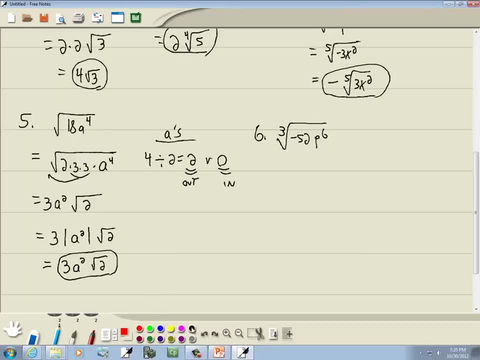 Remember, if you have a negative and you have an odd index, you can go ahead and bring that negative out in front. So I'm not even going to worry about that negative, just put it out in front. 52 is 2 times 26,, which is 2 times 13,. okay, times p to the 6.. 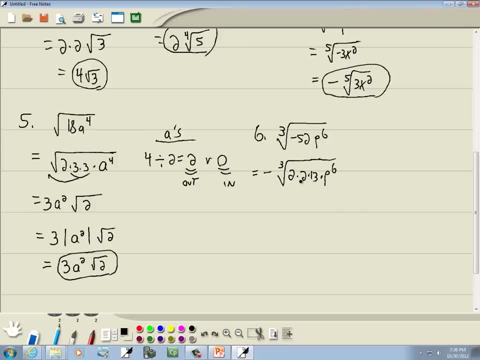 Well, our index is 3,. I'm looking for a set of 3 of something And, um, I don't see any 3 of any numbers here, So we can't do anything there but the p's. We're going to take our power, which is 6, divide by our index. 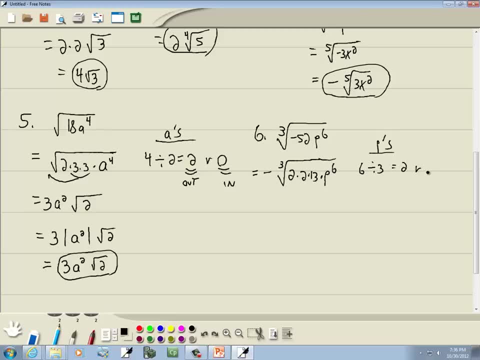 So 6 here divide by 3. That gives us 2 with a remainder of 0. This is how many come out and this is how many stay in. So we've got the negative out in front and, uh, we're going to have 2 p's come out and 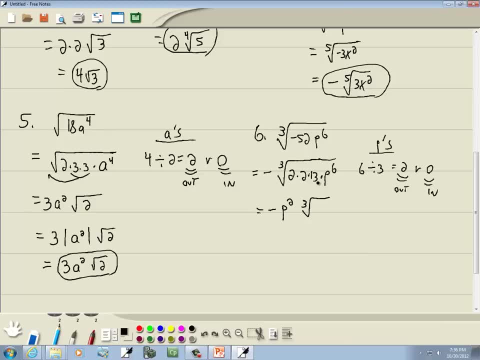 we're going to have 0 p's stay in And then 2 times 2 times 13 gives us 52. Okay, 52. And that's our answer. Now notice I didn't try to put absolute value bars around here. 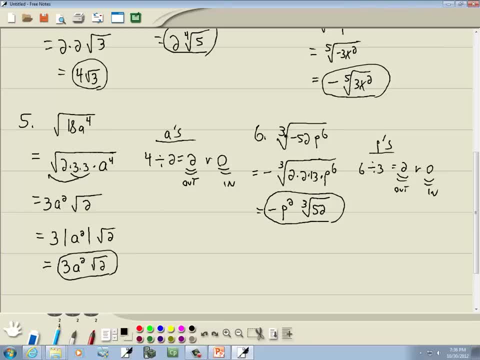 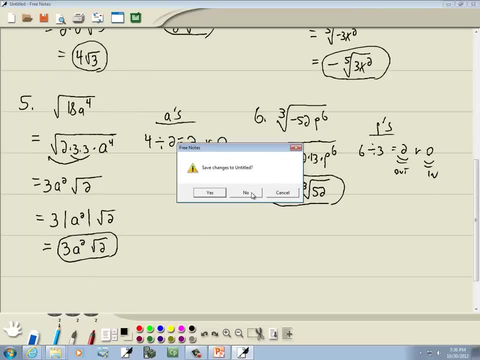 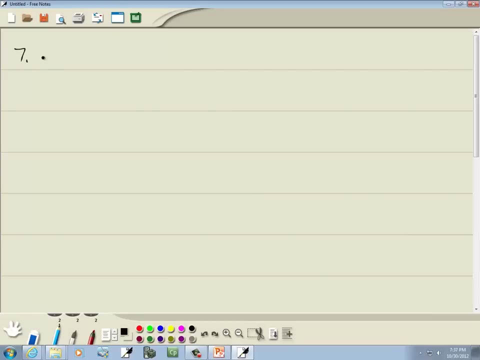 The only time you have to worry about the absolute value bars is when your index is even, and not when it's odd. Let me start a new page and let's look at our next problem. There's a lot of these problems, So we've got the square root of 50 m squared. 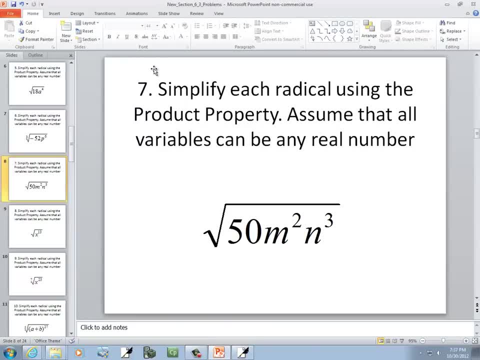 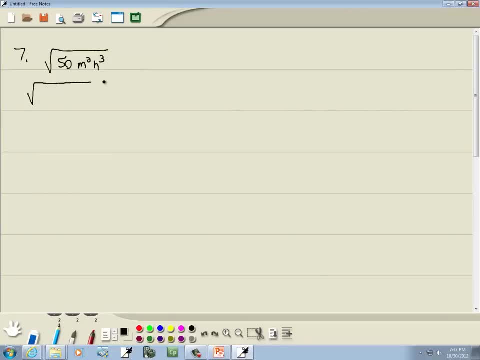 Into the third Instruction's still the same variables, or some of the old variables can be real numbers. Okay, First let's look at the numbers 50. Uh, that's 2 times 25, so 2 times 5 times 5.. 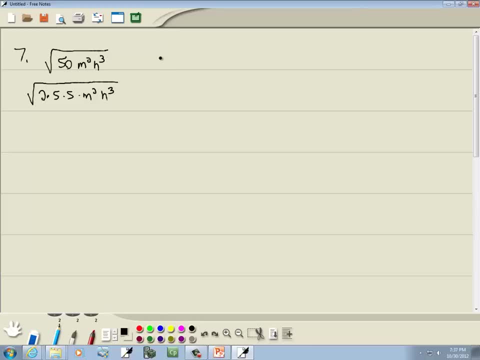 M squared into the third. Okay, So with our numbers, we're: this is a square root. it's, by default, 2 for the index. So we're looking for a pair of somethings. Here's a pair of 5's. 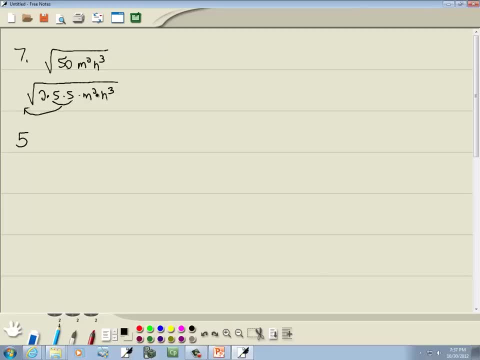 Those are going to come out as a single 5.. Now our m's. Let's figure out how many m's we're going to have come out. We're going to take our power. so which is 2, divide by our index. 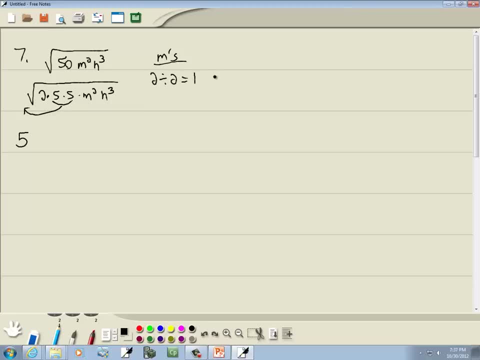 It's a square root, so it's, by default, 2.. So we're going to get: 2 divided by 2 is 1, with a remainder of 0. So this is how many come out and this is how many stay in. 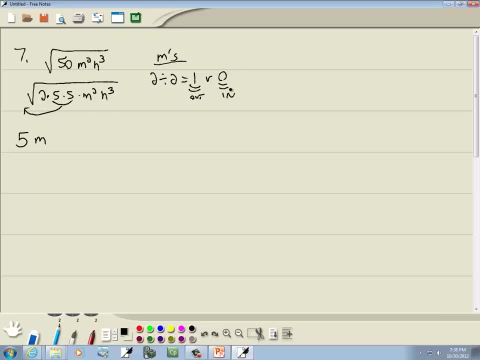 So we're going to have 1 m come out 0, 0 m. stay in Now n's. We got a third power there. so take 3, divide by our index. index for a square root again is 2.. 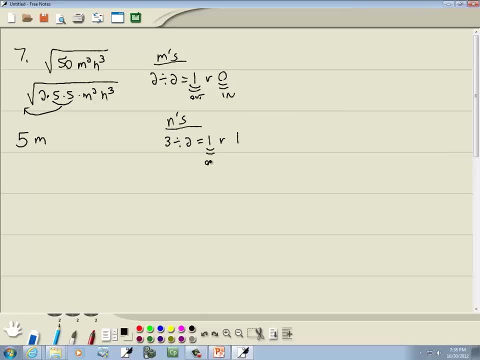 So we get 1 with a remainder of 1.. This is how many n's come out and this is how many stay in. So we're going to have 1 n come out Now. number wise, we still have that 2 in there. 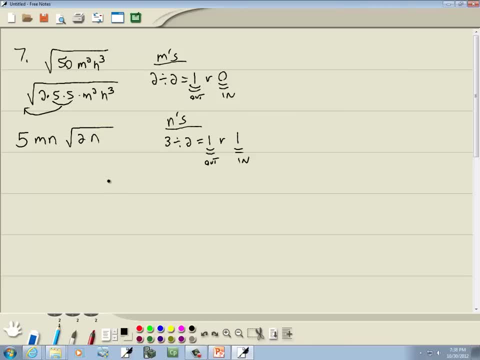 We have 0 m's and we have 1 n, So we'd have that Now. um, We cannot have a negative number. It's going to come out of a radical with an even index. So again we have to put absolute vibe bars around the mn. 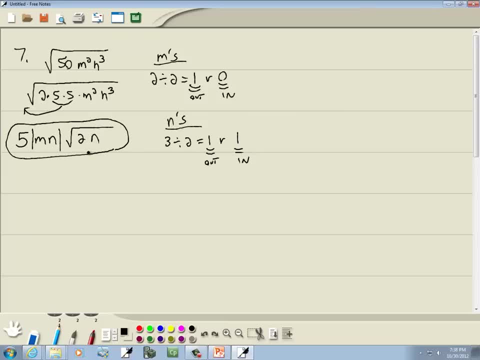 That'll ensure that whatever comes out is positive, and that's our answer, Number 8.. We've got the square root of x to the 13th. Well, for x's, take our power, which is 13,. divide by our index. 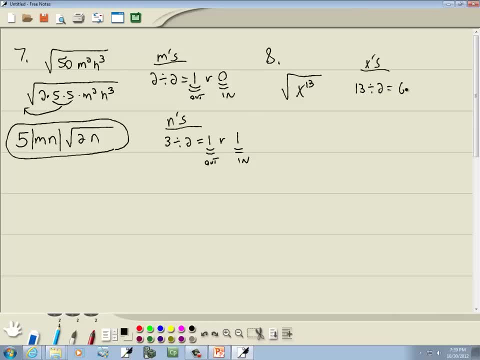 It's a square root, so it's, by default, 2.. So that gives us 6 with a remainder of 1.. This is how many come out. So we're going to have 6 x's come out and this is how many x's stay in. 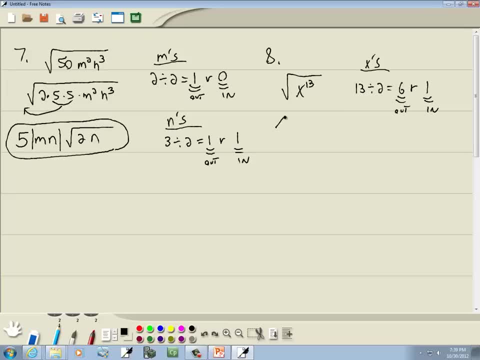 So we're going to have 1 x stay in. So we're going to have 6 x's come out and we'll have 1 stay in, Like that. Now again, we brought out a variable and you have to worry about the absolute vibe. 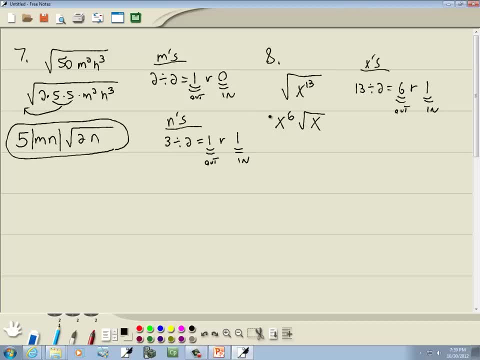 bars. We're going to bring out a variable from a radical with an even index. So we're going to put the absolute vibe bars here. But think what x to the 6th does. Well, actually, when you have x to any even power, it'll always become positive. 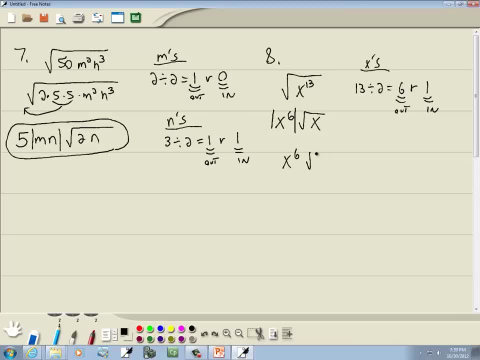 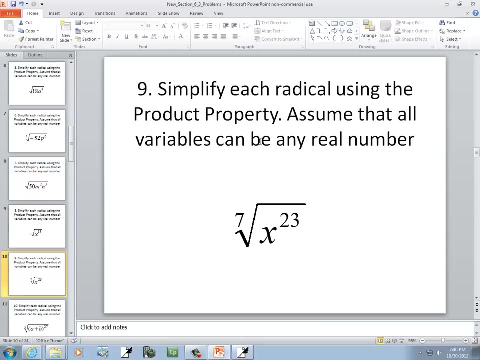 So those absolute vibe bars aren't necessary, so we'll go ahead and drop them, And this is our answer right here. Get a drink. Okay, Let's take a look at the next one. Get the index of 7,, x to the 23rd. 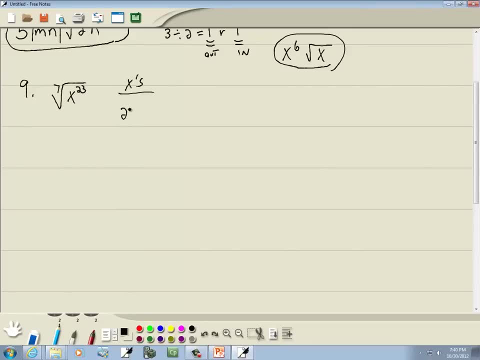 Well, again, we'll take our power, which is 23,, divide by our index, which is 7.. That gives us 3 with a remainder of 2.. This is how many x's come out. This is how many x's stay in. 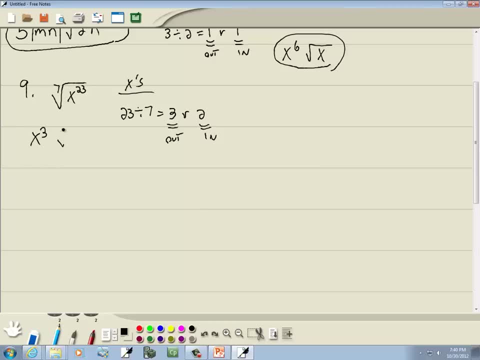 So we're going to have 3 x's come out and we'll have 2 x's stay in Now think: do we need to worry about the absolute value bars? No, because the index is odd. The only time you have to worry about the absolute value bars is when the index is even. 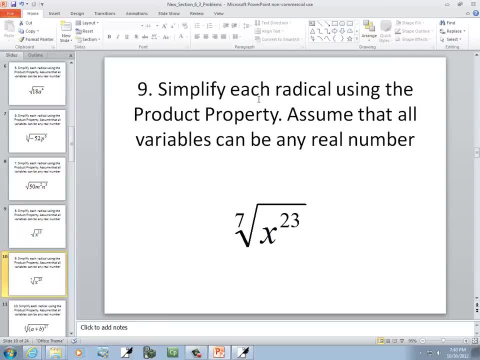 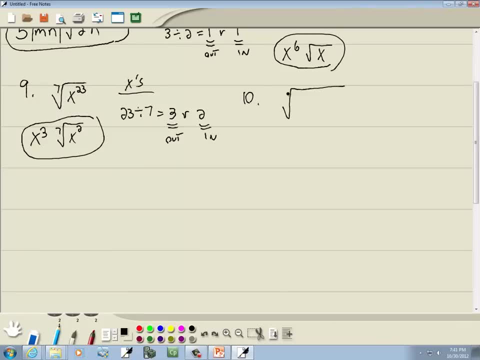 So that's our answer. Okay, let's look at this one: Get the 5th root, Get the 27th root of a plus b, 27th power. Doesn't matter what we're talking about Here. we're talking about a plus b's. 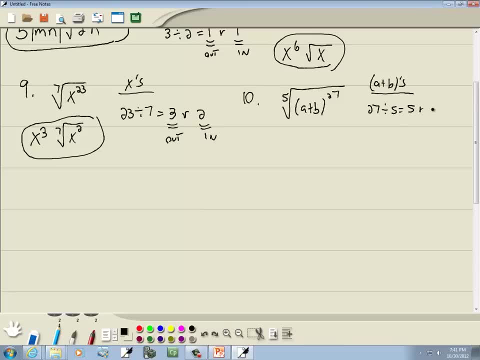 So we're going to take our power, which is 27,, divide by our index, which is 5.. That gives us 5 with a remainder of 2.. So this is how many come out and this is how many stay in. So we're going to have 5 a plus b's come out, And we're going to take our power, which is 27, divide by our index, which is 5.. That gives us 5 with a remainder of 2.. 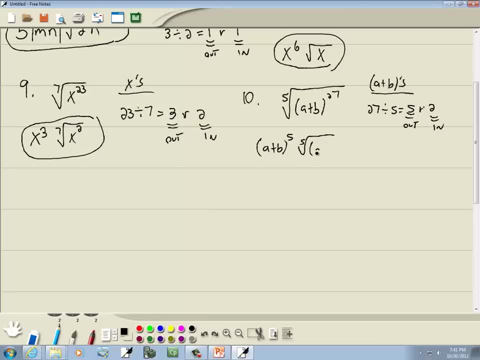 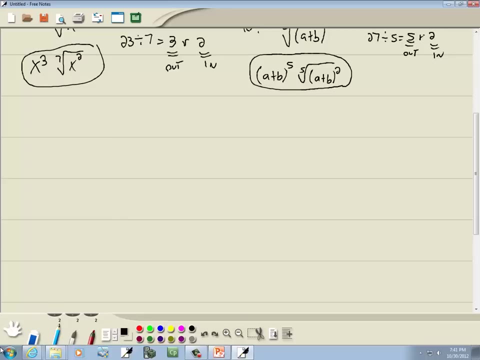 And we'll have 2 a plus b's. stay in. Now our index is odd, so we don't need to worry about the absolute value bars, And that's our answer. This one's kind of a specific type and we'll talk more about it after we work one. 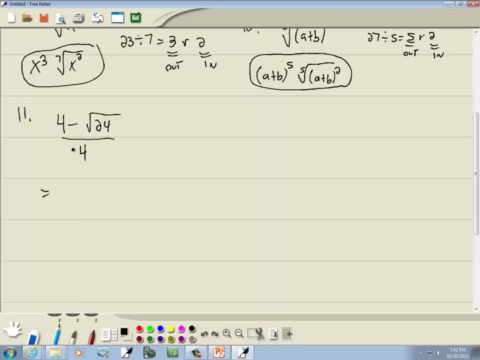 No matter where you are in math, if you can simplify your radicals, you should Square root of 24, I can simplify, So I've got: 4 minus 24 is 2, 4, 8 times 3.. So that's prime factorization. 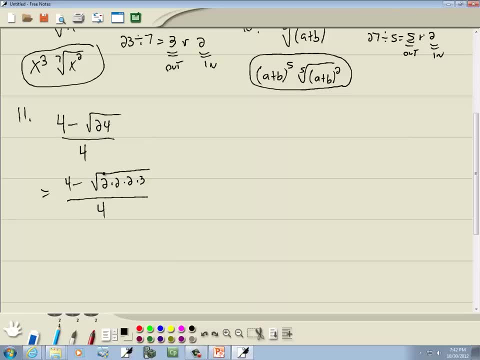 Now, this is a square root, so our index is 2, so we're looking for a pair of somethings. Here's a pair of 2's, so that's going to come out in front as a single 2.. So we've got 4 minus 2, and then we're left with 2 times 3 inside, which is 6.. 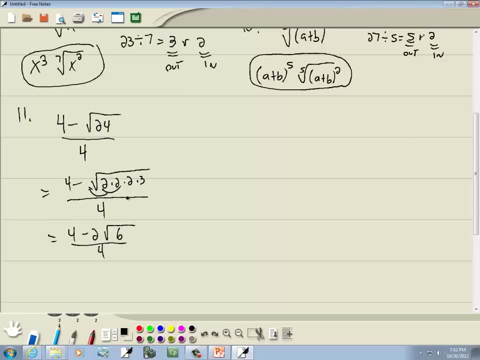 We can only bring something out if it's a pair, like a pair of 2's, a pair of 3's. Now, this type of form you see right here. you see this a lot in the quadratic formula which we'll see later in this course, and then you'll see it in college algebra 2.. 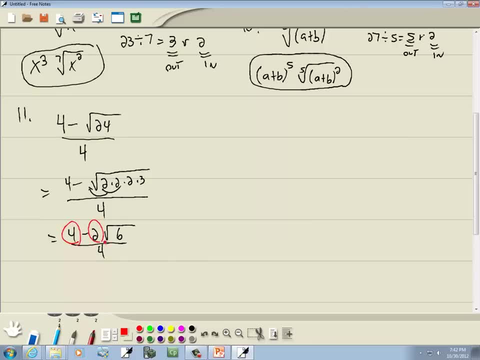 And basically it says: if you can divide this number and this number and this number by the same number, do so. Well, those are all divisible by 2.. So 4 divided by 2 is 2.. 2 minus 1 square root of 6 over 2, which gives us 2 minus square root of 6 over 2.. 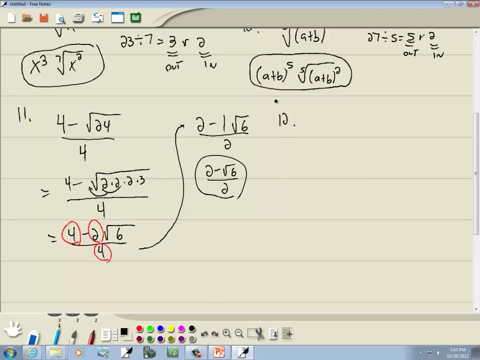 And that's our answer. Let's look at another one of those 12 minus square root of 48 over 24.. Again, no matter where you are in math, you should simplify your radicals before you go on. So we've got 48.. 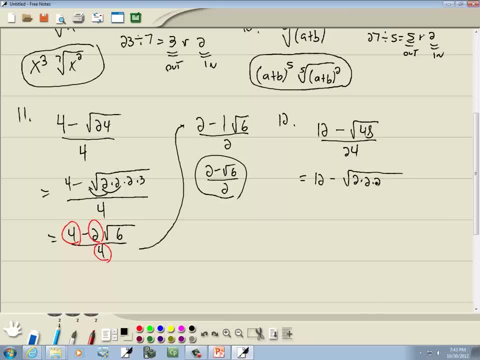 Uh, 48.. Is 2 times 2, 2,, 4,, 8,, 16,, 48.. 2, 4,, 8,, 16,, yeah, 48.. Okay, we're looking for a pair of somethings. 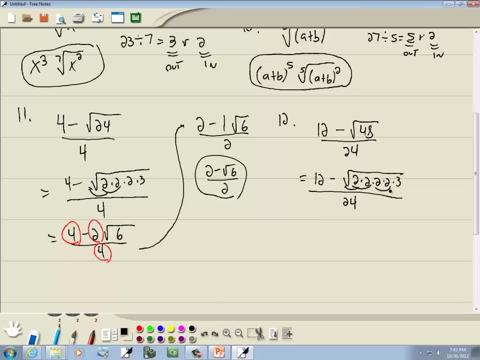 Now, here's a pair of 2's. those are going to come out. Here's another pair of 2's those are going to come out. Now, when they come out, they come out with multiplication between them. So I'll have 2 times 2 in front of the square root and then a 3 over 24.. 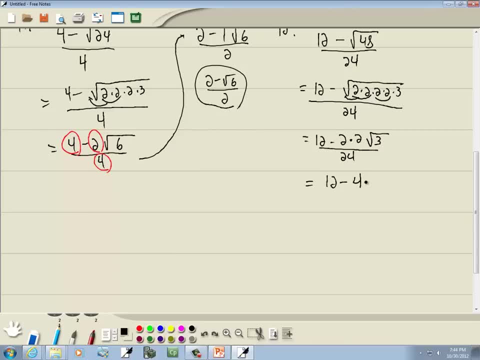 12 minus 2 times 2 is 4.. Again, they should call this the 3 number rule or something. But if you can divide this number, this number and this number by the same number, do so. And those are all divisible by 4.. 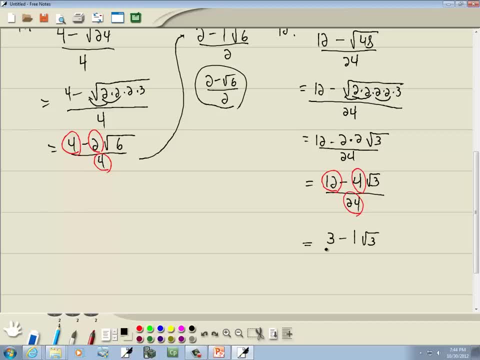 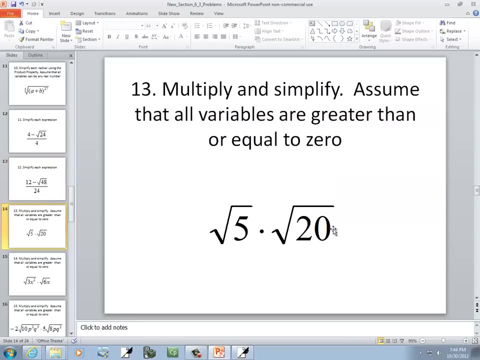 12 divided by 4 is 3 minus 1 square root of 3 over 6.. Which gives us 3 minus square root of 3 over 6.. And that's our answer. Okay, now let's look at this one. 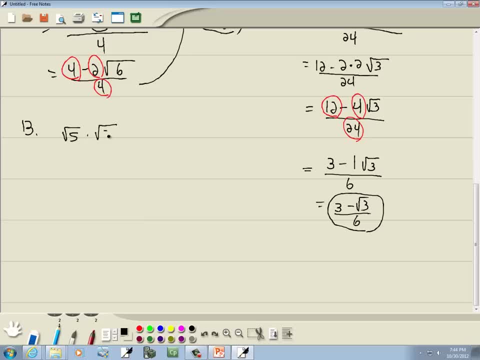 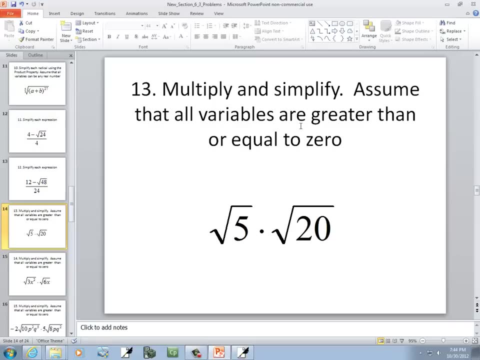 And this one I got square root of 5 times square root of 20.. Again we're back to the product rule here. It says: multiply and simplify. Assume that all variables are greater than or equal to 0.. Assume that all variables are greater than or equal to 0.. 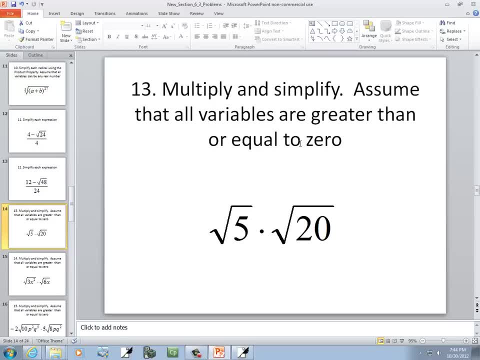 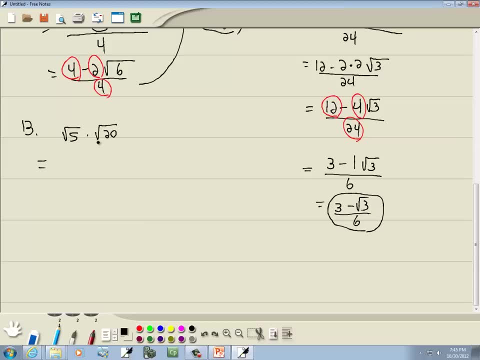 What they're telling you there is it's all. variables are positive, So we don't need to worry about absolute value bars in any problem. we bring out a variable. Okay, so multiply these two together. As long as the index is the same, you can put them underneath the same radical. 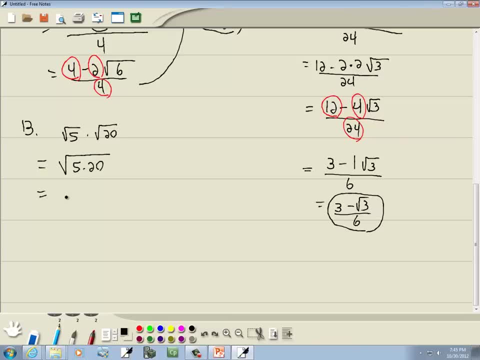 Multiply together. Now, you don't want to actually multiply them together, though. The reason why is you want to see what can simplify. 20 is 5 times 2 times 2. That's prime factorization 20.. Now, after I do that, this 5 just carried down. 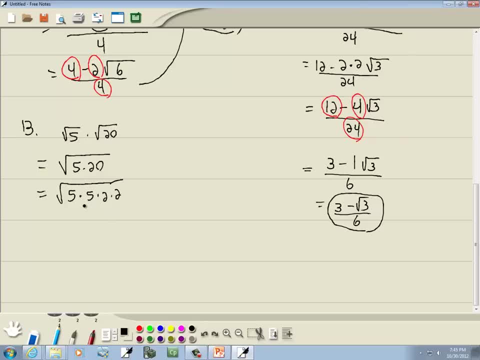 And then this 20 is the 5 times 2 times 2.. Remember The square root. we're looking for pairs of something. Here's a pair of 5s Those are going to come out as a single 5.. 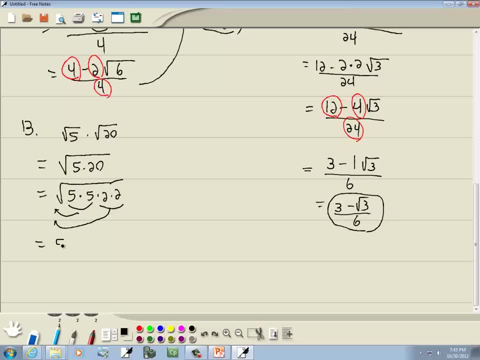 Here's a pair of 2s Those are going to come out as a single 2.. Now again, when they come out, they come out with multiplication between them And there's nothing left inside the square root. so we drop it. 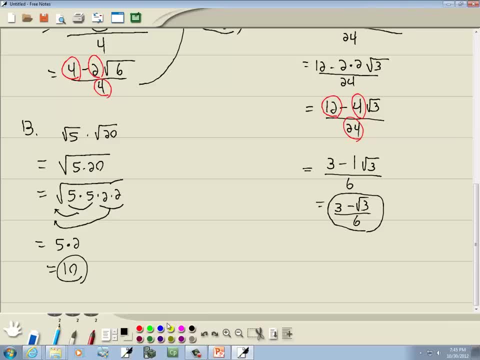 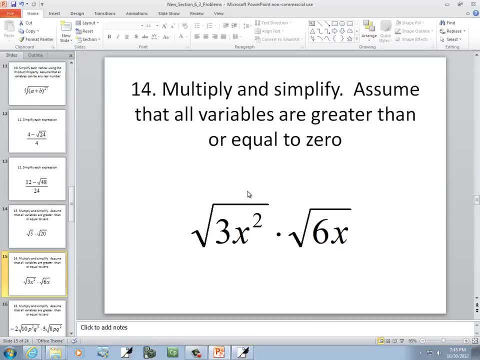 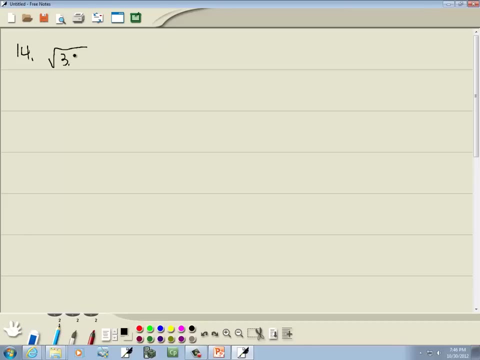 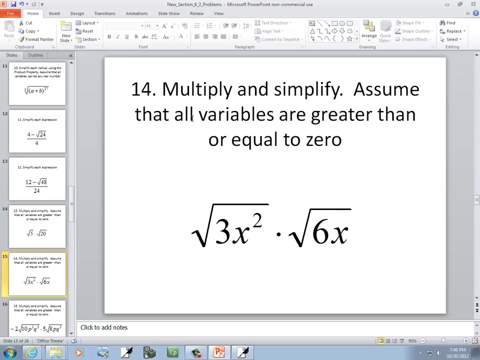 So 5 times 2 gives us 10.. Let's start a new page. Let's look at the next problem. We've got square root 3x squared times the square root of 6x And again it says: assume all variables are greater than or equal to 0.. 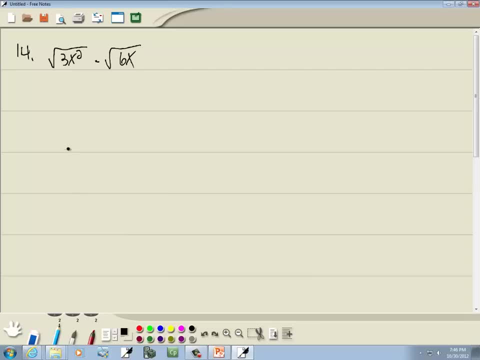 So, anything that comes out, we don't have to worry about the absolute value bars. Well, the indexes are the same. We're multiplying these together, So we'll multiply what's underneath them And I'll put the numbers together. So I've got 3 times 6.. 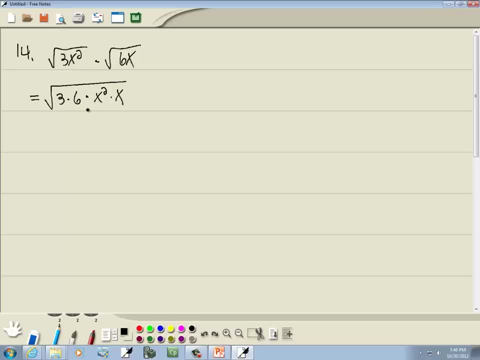 And I'll put the x's together. So x squared times x, Well, 6 is 3 times 2.. And x squared times x gives us x to the third. Now, remember we're looking for a pair of somethings. 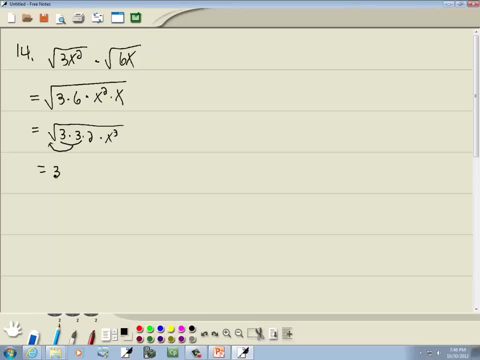 Here's a pair of 3s Those are going to come out in front as a single 3.. Now the x to the third. Let's talk about the x's Again. we'll take our power, which is 3.. 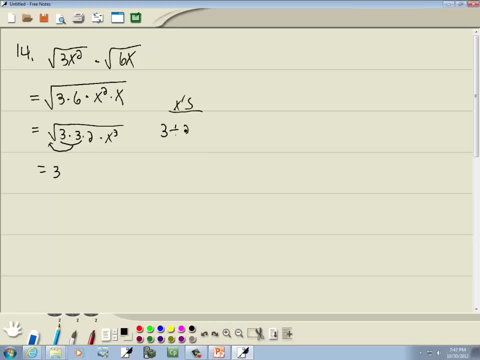 And you divide by your index, And this is a square root. so again it's 2.. And this is old-style division: 3 divided by 2 is 1 with remainder of 1.. This is how many x's come out. 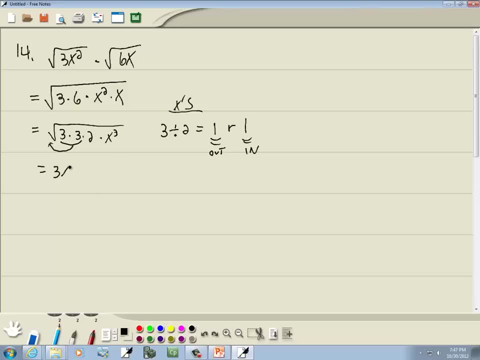 This is how many stay in. So we're going to have 1x come out And we're left with the 2 inside And we said there's 1x left inside. Now, normally I'd have to worry about the absolute value bars on that. 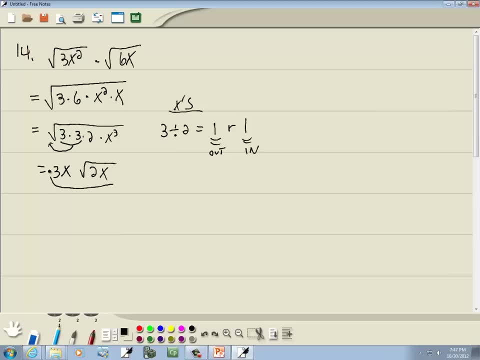 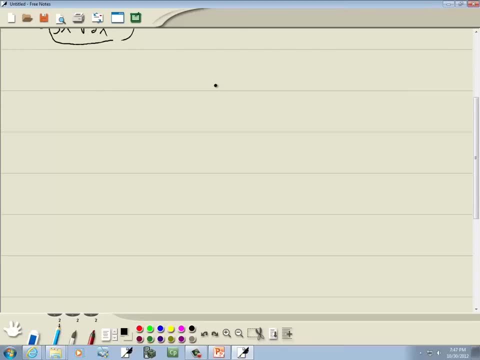 But this says: assume that all variables are greater than or equal to 0. So we don't need to worry about that And that's our answer. Let's go down here. Here we got negative 2 square root of 10p squared q to the fifth times 5 square root of 8p squared. 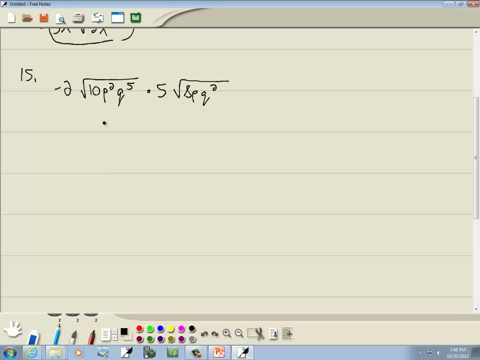 Now, if you're multiplying radicals together, you multiply what's underneath them, assuming the indexes are the same. If you have numbers out in front, you multiply those numbers together. So negative 2 times 5 gives us negative 10. And we'll multiply these together. 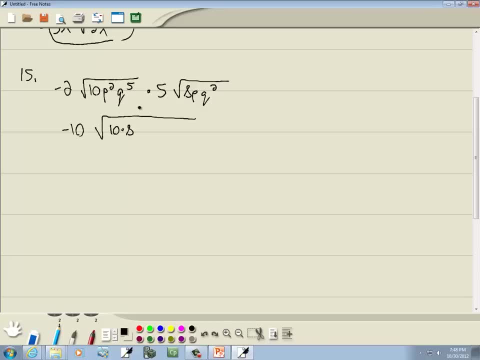 And I'll put the numbers together. So I got 10 times 8.. I'm going to put the p's together. So I got p squared p, And I'll put the q's together. So I got q to the fifth q squared. 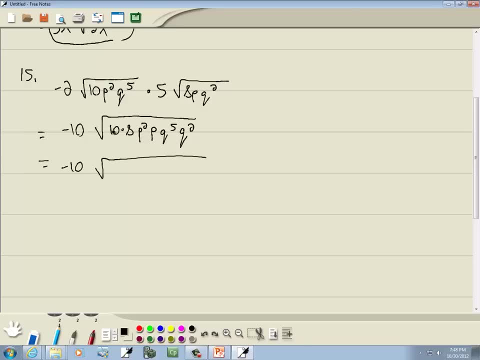 I want to do the prime factorization. 10 is 5 times 2.. 8 is 2 times 2 times 2.. p squared times p gives us p to the third, q to the fifth times q squared gives us q to the seventh. 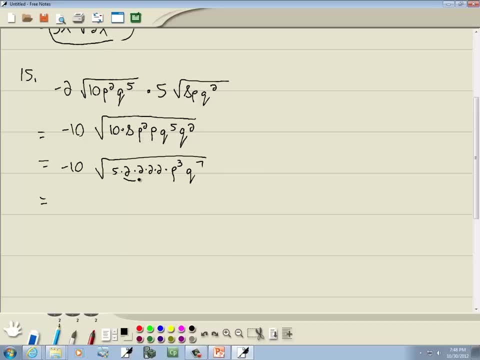 Now, this is a square root, so we're looking for a pair of somethings. Here's a pair of 2s That's going to come out, And here's a pair of 2s That's going to come out. 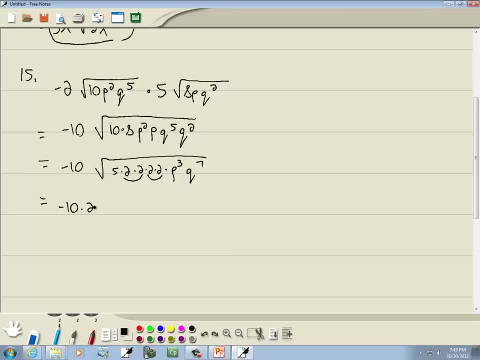 Now, when they come out, the first pair of 2s comes out as a single 2.. Second one comes out as a single 2.. And they're multiplied by what's already out in front. Now for the p's. 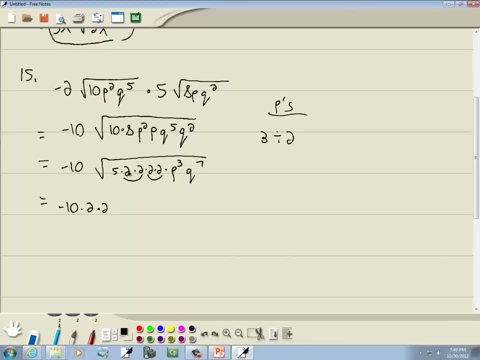 My power is 3.. Divide by my index, It's a square root, so it's, by default, 2.. 3 divided by 2 gives us 1 with remainder of 1.. So this is how many p's come out. 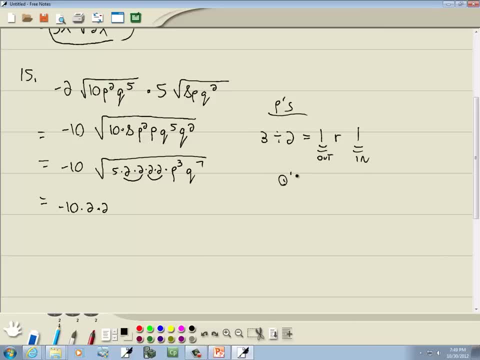 And this is how many p's stay in. Now for our q's. Take our power, which is 7. Divide by our index, which is still 2.. So we get 3 with remainder of 1.. And again, this is how many come out. 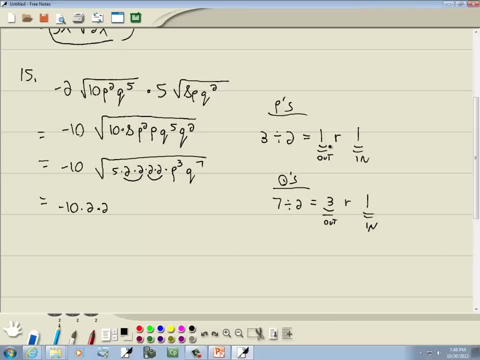 And this is how many stay in. Okay, so we're going to have 1p come out. We're going to have 3q's come out. Okay, those 2s are gone. We're left with a 5 inside. 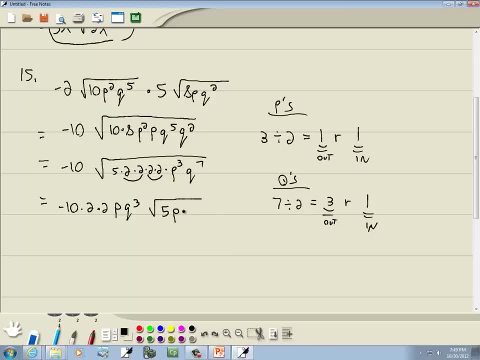 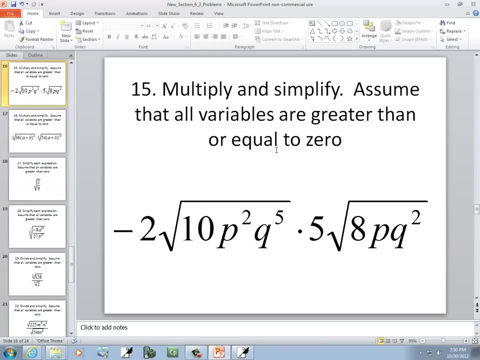 We have 1p left inside And we have 1q left inside. Now again, the instructions are: assume all variables are great, They're greater than or equal to 0. So we don't need to worry about absolute value bars. 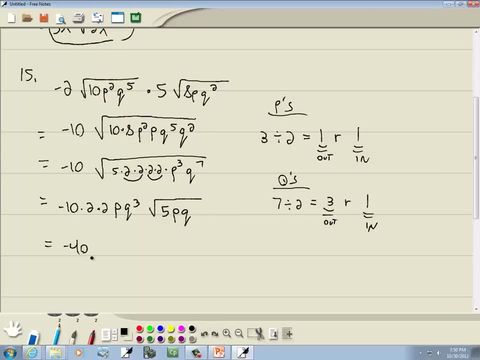 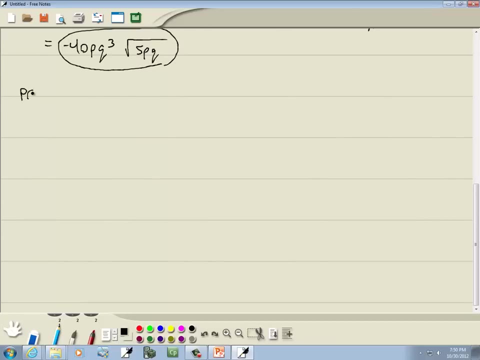 2 times 2 is 4.. Times negative 10 is negative 40. pq to the third square root of 5pq And that's our answer. Okay, We've got some more properties Now here. If you've got the, whatever your index might be. 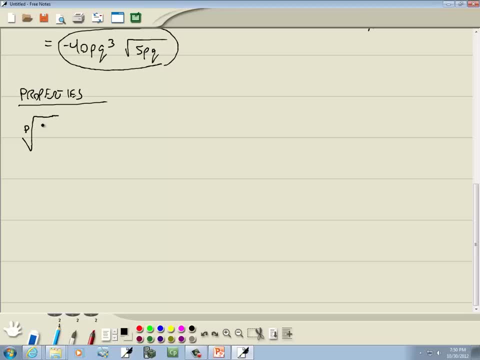 I would use i, but i's are kind of hard to see. If you've got division, You've got the radical of. I don't remember what variables I used. I think they were m and n, So you've got the radical of m over n. 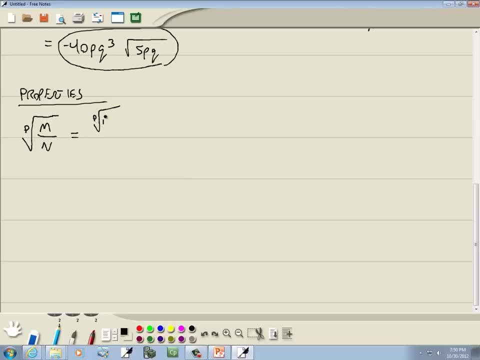 Then you can split it up. Put a radical around top And you can put a radical around the bottom. Now your index stays the same. That doesn't change. You can just split them up. Now you can go this direction or you can go that direction. 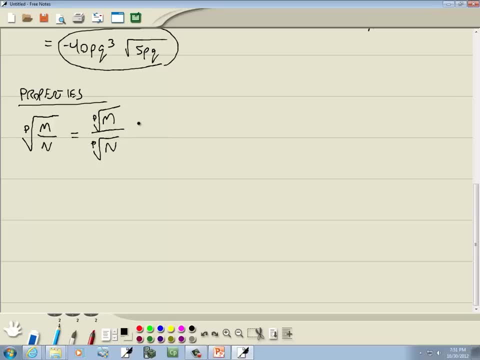 So that's when we're talking about division And for simplifying radicals In terms of fractions. so simplifying radicals in terms of fractions, first thing is: no fractions inside of a radical, so no fractions inside of a radical. and second thing is: no radicals in the dominator. 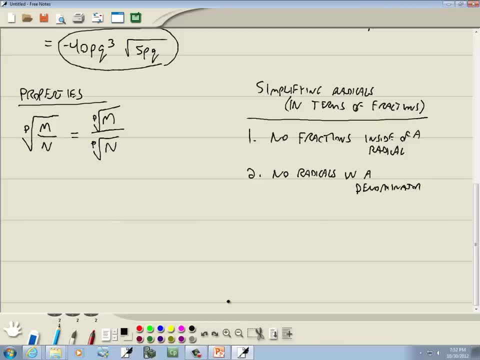 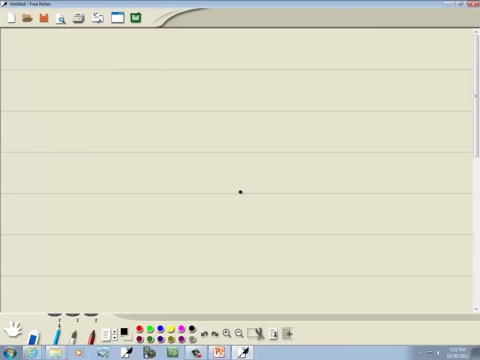 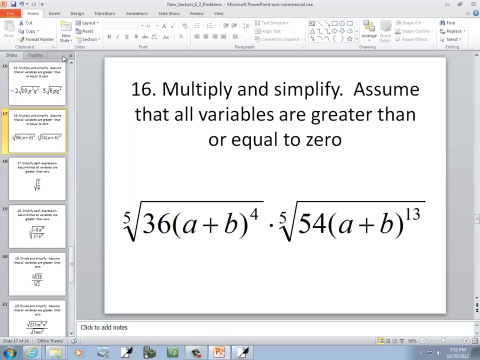 so no radicals in denominator. so when working in problems, we want to keep that in mind. nope, we got another multiplication. my eyes are, eyes are getting off. let's go and do this one and then we'll look at those, those properties, okay. fifth root of 36 times a. 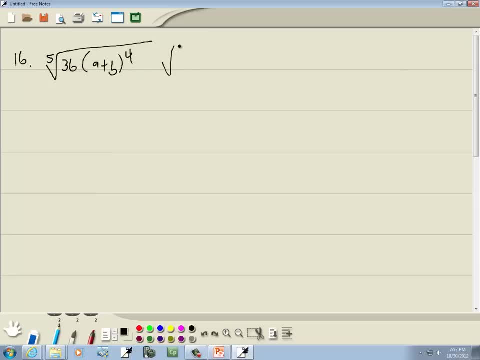 plus B to the fourth times, the fifth root of 54 times a, plus B to 13th. well, we're multiplying two radicals together, so put them into a single radical fifth root and we'll have 36 times 54 and we'll put the a plus B's together, so we've got a plus B to the fourth and a. 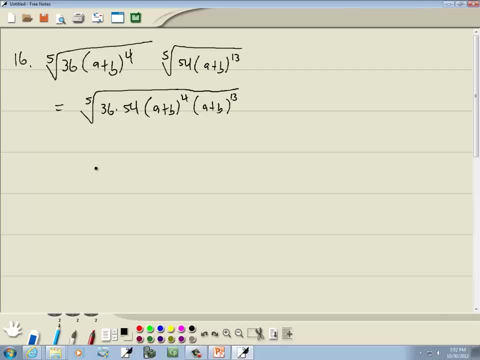 plus B to the thirteenth. now 36, 2 times 18, 2 times 2, 4, 2, 4, 12, 36, 54, that's 2 times 3. well, 3, 9, 27, 54. okay, I did prime. 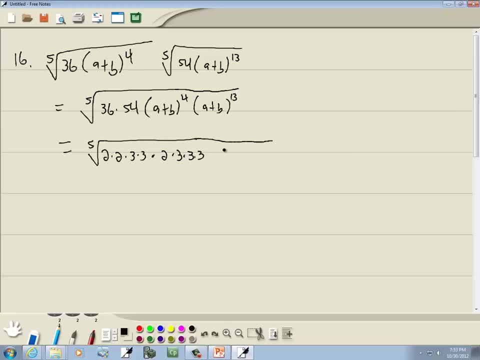 prime factorization, 36 and prime factorization and 54. now a plus B to the fourth times, a plus B to the 13th. you add the exponents, so you got a plus B to the 17th. okay, now we're looking for our 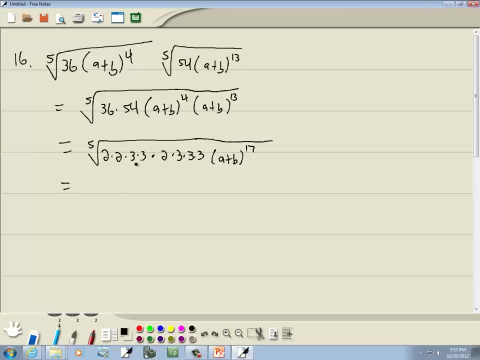 index is 5, so looking for set up five something. well, we have two trees there and three-threes here. we got 53 total, so those gonna come out in front as a single three. that twos I can't do anything with this is only three of them. 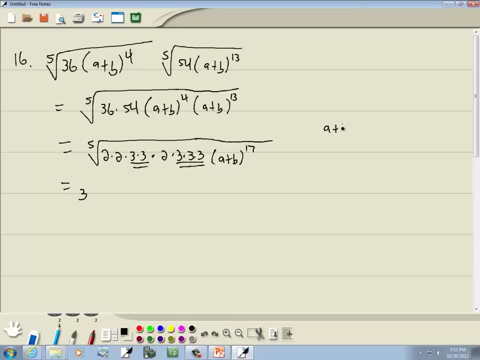 Now the a plus b's. Again, we take our power, which is 17,, divide by our index, which is 5,, and that gives us 3 with a remainder of 2.. This is how many we have come out and this is how many we have stay in. 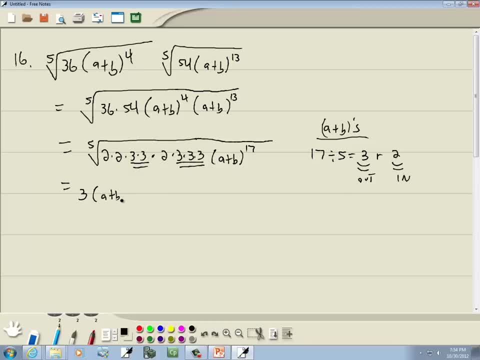 So we're going to have a plus b to the third power and inside we said we had the 2's remaining 2 times 2 times 2 is 8, and we have 2 a plus b's. So we've got a plus b to the second power and that's our answer. 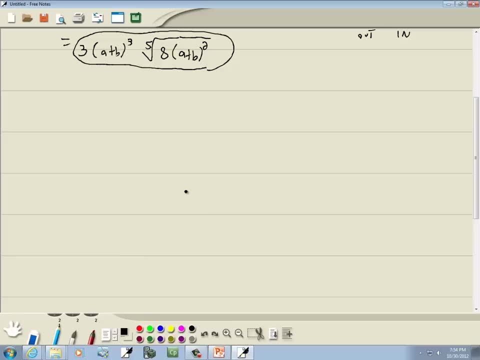 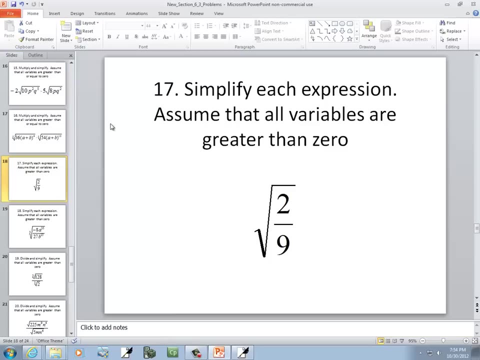 Okay, now let's look at division. So we've got square root of 2 ninths. It says: simplify each expression. assume all variables are greater than 0.. Assume that all variables are greater than 0.. They're telling you: don't worry about absolute value bars when you have variables. 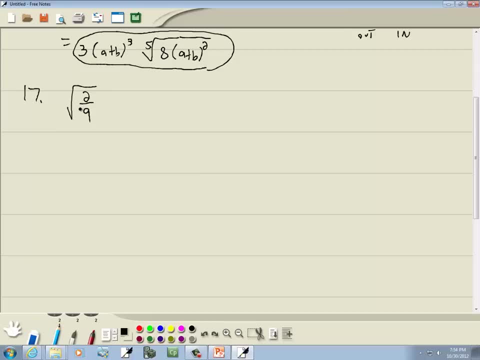 Well, we can't have a fraction inside of a square root. We can't have a fraction inside of a radical. we said Our property says we can split this up. You can put a square root around the top and a square root around the bottom. 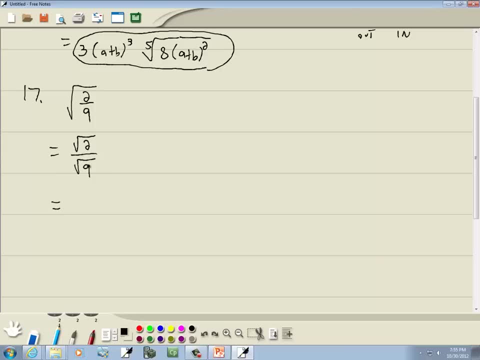 Well, that doesn't seem to do us any good, because we said we can't have a fraction inside of a radical, We can't have a radical in the denominator, But in this case, square root of 9, 9 is 3 times 3.. 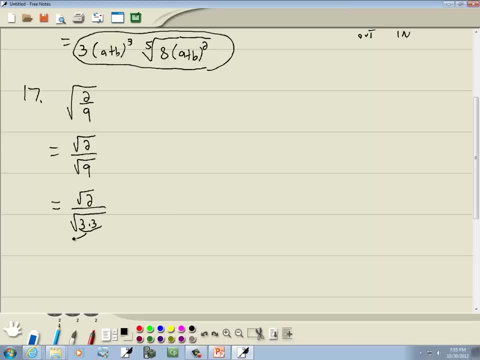 With a square root. we're looking for a pair of somethings, Here's a pair of 3's, so those are going to come out as a single 3.. So our answer is square root of 2 over 3.. 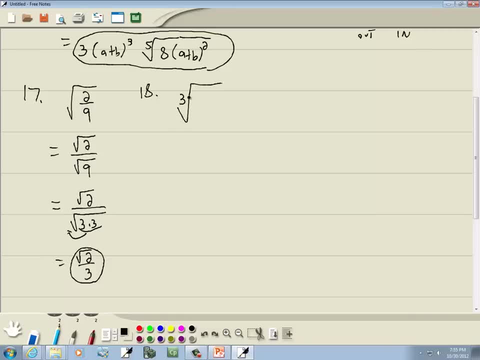 Number 18.. We've got the cube root of negative 8.. A to the 33rd, over 27,, b to the 15th. Well, we said we can't have a fraction inside of a radical, so that's the main problem here. 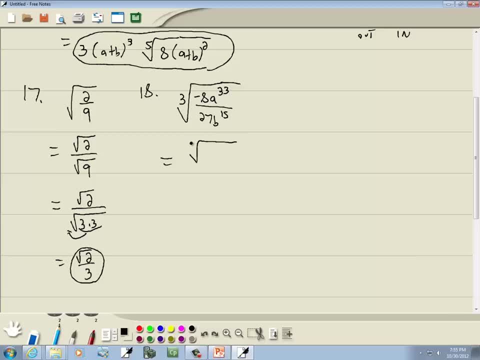 Our property allows us to put a radical around the top. So we've got the cube root of negative 8, a to the 33rd, and then we put a cube root around the bottom, We've got 3. 27, b to the 15th. 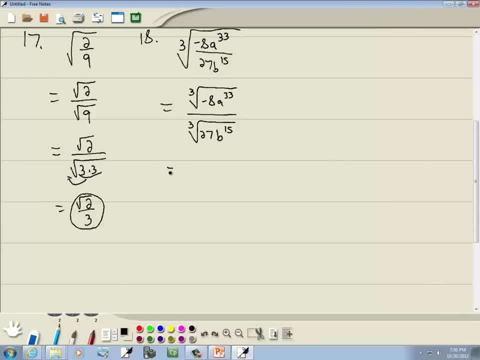 Now, by breaking this up, we can focus on each piece separately, And that helps a little bit. Now, up on top, our index is odd and we've got a negative number. Remember we said we can just take negatives and bring them out of the radical. 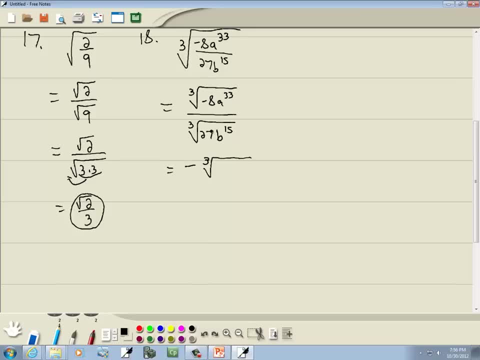 assuming your index is odd. Now 8 is 2 times 2,, well, 3, 2's. And then we've got 8 to the 33rd. On the bottom, 27 is 3, 3's. b to the 15th. 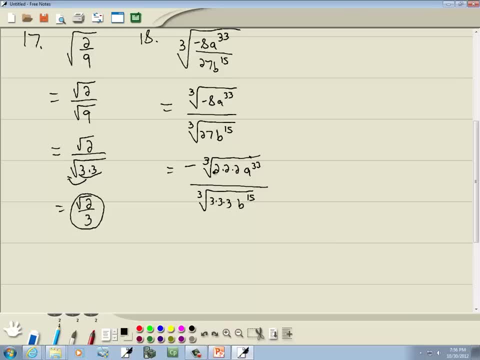 Well, our index is 3,, which means we're looking for a set of 3 of something. Here's 3- 2's, so those are going to come out as a single 2.. And down below we have 3- 3's. 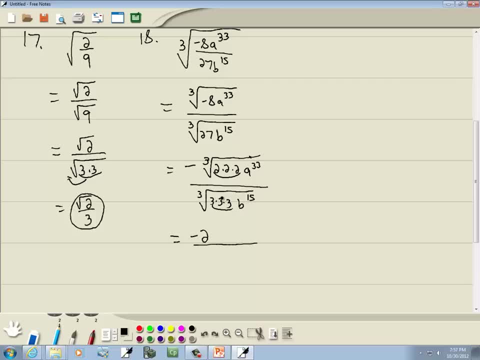 So again, our index is 3.. We're looking for a set of 3 of something. Those set of 3 3's can come out as a single 3.. Let's look at our variables now. the a's: 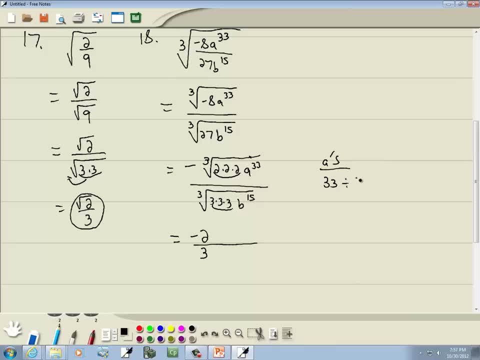 We'll take our power, which is 33, divide by our index, which is 3,, the number in the slot here. that gives us 11 with a remainder of 0. This is how many come out and this is how many stay in. 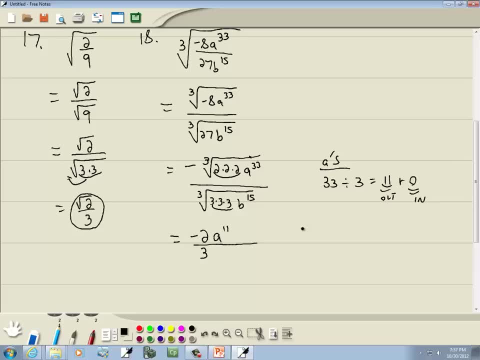 So we're going to have 11 a's come out Now in this one, the b's, We take 15, divide by 3.. 3, 3's, 3, 3's: This is 5 with a remainder of 0.. 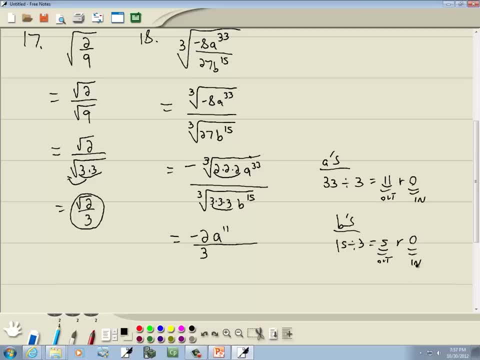 So we're going to have 5 b's come out and we'll have 0 b's remain in. So we're going to have 5 b's come out and there's no b's left inside. So actually our radicals both disappear. 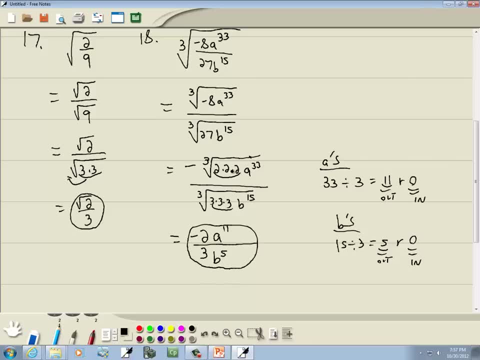 Now, in this case, by using that property, it allowed us to break them into smaller pieces so we could work each one and have it a little bit easier than this whole mess right here Over here. it allowed us to, even though we couldn't simplify the top part. it allowed us to get rid of the 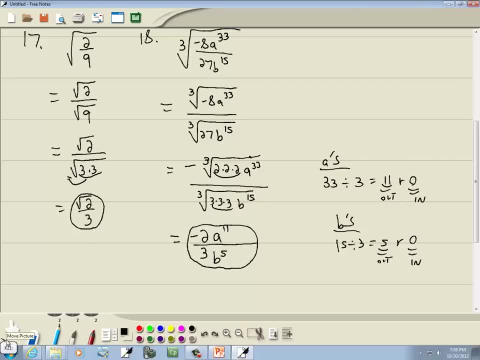 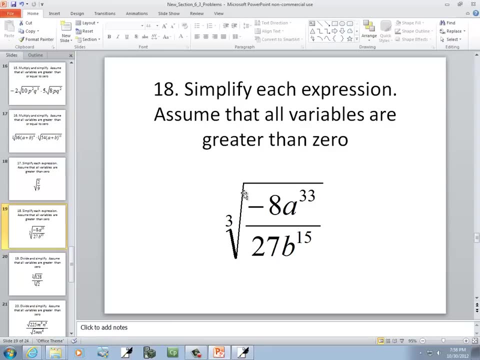 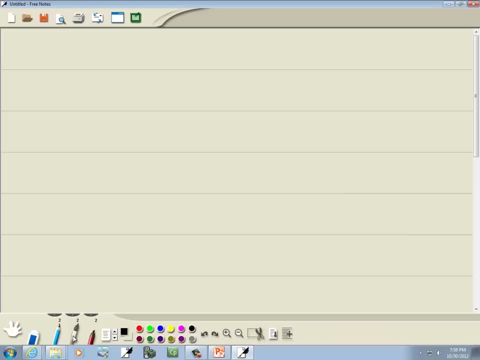 the fraction inside of radical. by doing that, Let me start a new page. Let's take a look at this one. We've got the cube root of 128 over the cube root of 2.. Well, the main problem here is we can't have a radical in the denominator. 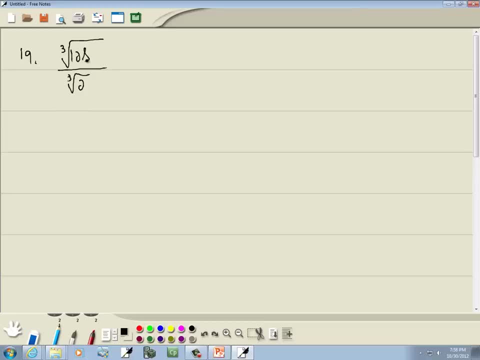 Now there's nothing. I can really simplify The top part. I can simplify a little bit, but we could merge this back into a single radical putting a fraction together, So 128 over 2.. You can go both directions on your formula. 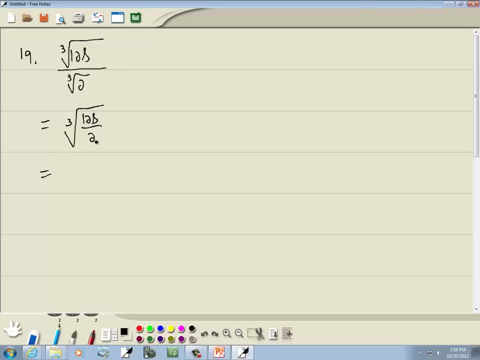 Why would we do that? Well, because I could see that 128 is divisible by 2.. So this, This becomes the cube root of 64.. If I did a prime factorization of 64, that's 2 times well, 6, 2s. 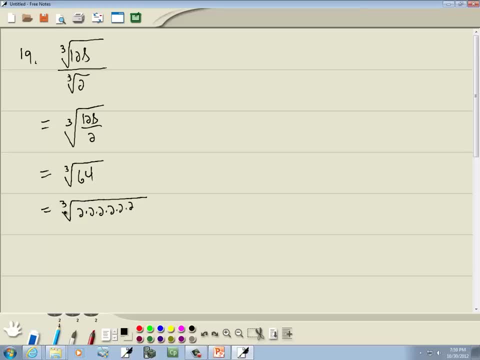 2,, 4,, 8,, 16,, 32,, 64.. Now our index is 3,, which means we're looking for a set of 3 of something. Here's 3, 2s. Those are going to come out as a single 2.. 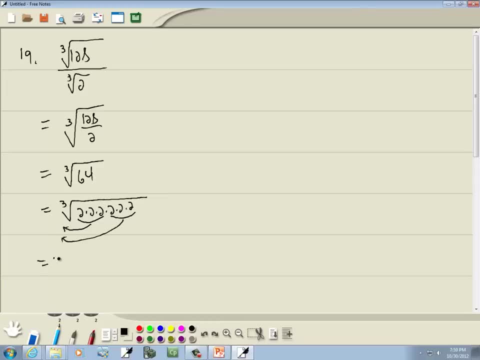 And here's 3, 2s. Those will come out as a single 2.. Now, when they come out, they come out with multiplication between them. Now, there's nothing left in the middle. Now, there's nothing left in the middle. 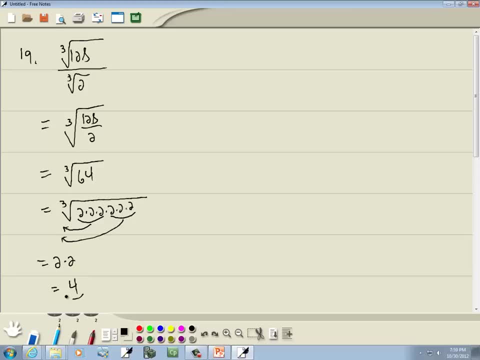 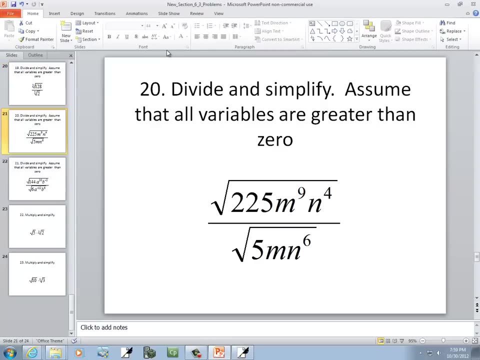 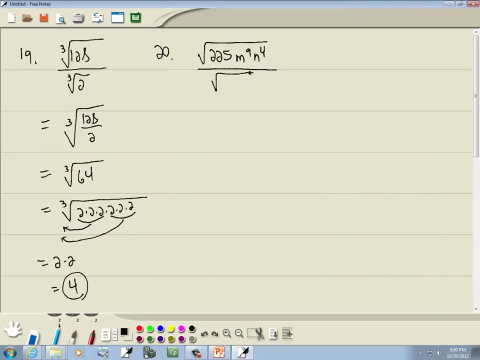 Now there's nothing left in the middle. We've got one side of a radical, so it disappears, and 2 times 2 gives us 4.. Let's take a look at this one. We've got square root of 225 into the 9th, into the 4th, over square root of 5m into the 6th. 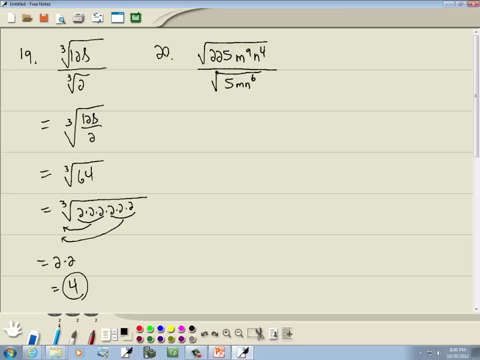 now, sometimes, of course, the main problem is here we can't have a radical in the denominator. but sometimes you can see that if you have radical on top and radical on the bottom, that if you merge them together they would simplify a little bit. and that's what this looks like. 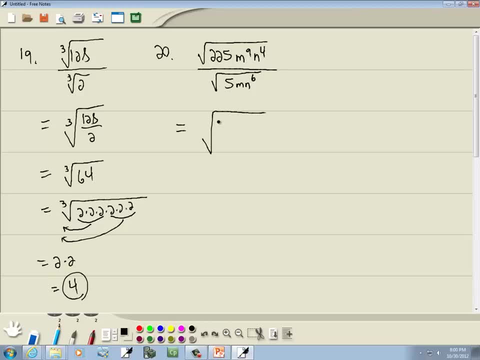 so let's go ahead and temporarily put them together. sometimes you temporarily put them together, you simplify and then you break them back apart, as weird as that seems. ok, I put them together. I got 225 divided by 5. I have no clue what that is, but let me see. 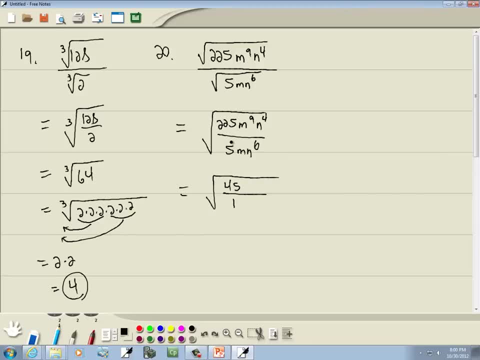 that's 45. now, here we have m to the power over m to the power, and this is like the first power. if I were to put an exponent there, it would be a 1. remember, if you have m to the power over m to the power, you subtract a smaller exponent. 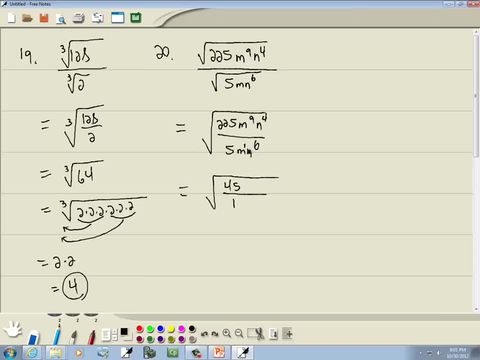 from a larger one, 9 9-1 gives you 8 and you're going to have m to the 8th where our larger exponent was, which is on top. now the n's. I got n to the 4th over n to the 6th. 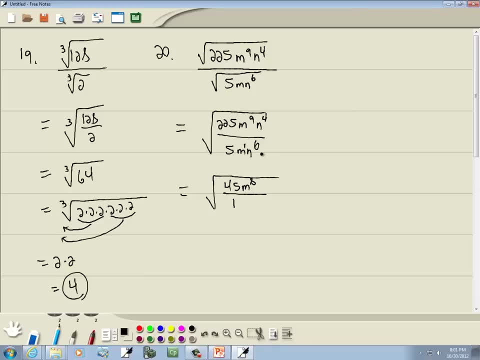 I'm going to subtract a smaller exponent from a larger one. 6-4 gives you 2, and you're going to have n squared where the larger exponent was, which was downstairs. so we're putting it in the denominator. ok, that's as much simplifying as we can do. so let's split them back apart. 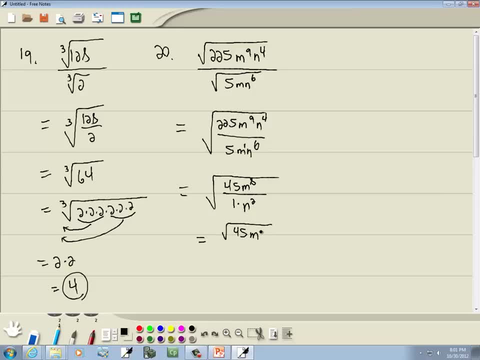 so we're going to put the square root of m to the power over m to the power, and we're going to put the square root of n to the 4th over m to the power. so we're going to put the square root of n to the power. 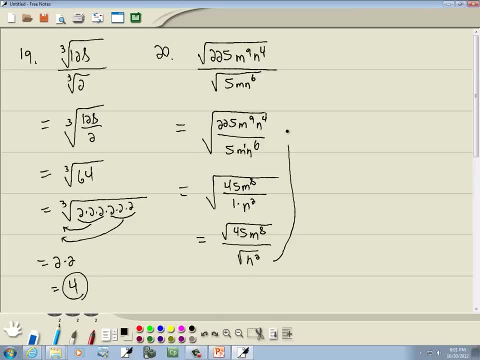 and we'll put a square root around the bottom. and we'll put a square root around the bottom, now the top part. I'm going to write that number, the prime factorization of that number, that's 3 times 3 times 5 m to the 8th over square root of n squared. 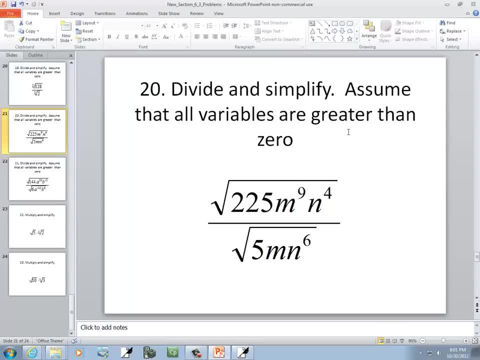 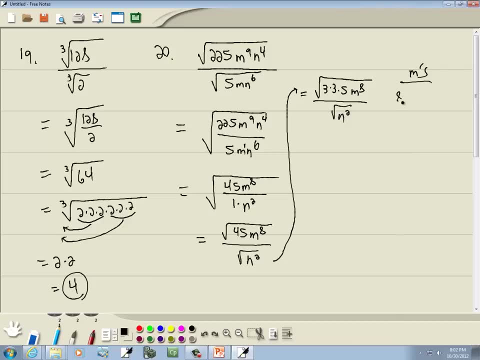 now our answer is say: assume that all variables are greater than 0, so we still don't need to worry about absolute value bars. so let's look at the m's. take my power, which is n, squared, which is 8, divided by my index. 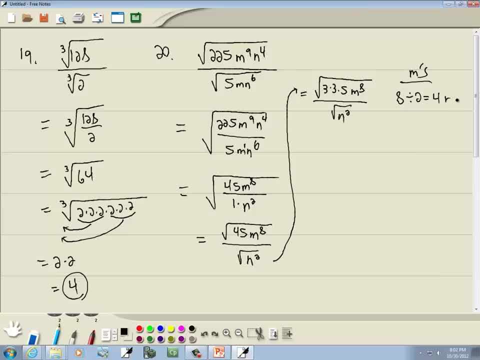 It's a square root, so it's default 2.. So that gives us 4 with a remainder of 0. This is how many m's come out. We're going to have 4 m's come out and this is how many stay in. 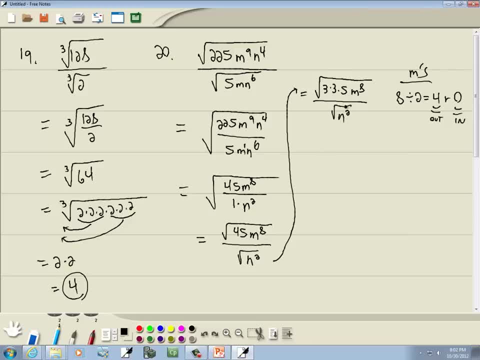 So we're going to have 0. stay in. Now. this is a square root, so we're looking for a pair of numbers or a pair of somethings. Here's a pair of 3's, so those are going to come out as a single 3.. 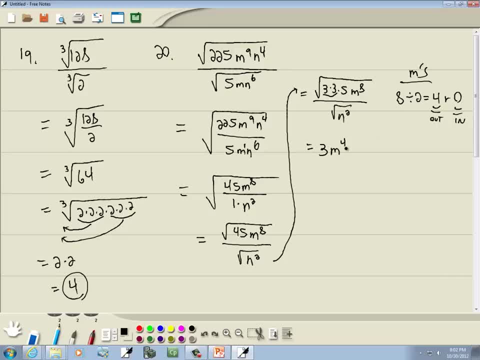 Now we said we have 4 m's come out And we're left with a 5 inside, like that. Excuse me Now the n's, Our power, is 2, divided by our index, which is 2.. 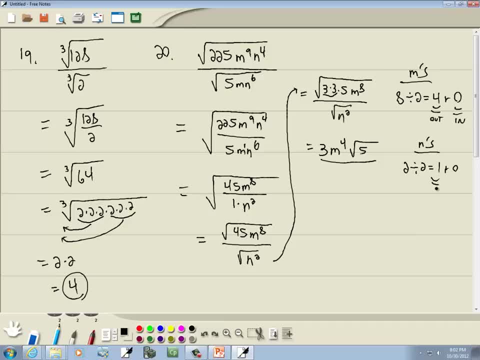 That gives us 1 with a remainder of 0.. This is how many come out. so we have 1 n come out. And this is how many stay in. so we have 0 n stay in. So we have 1 n come out. 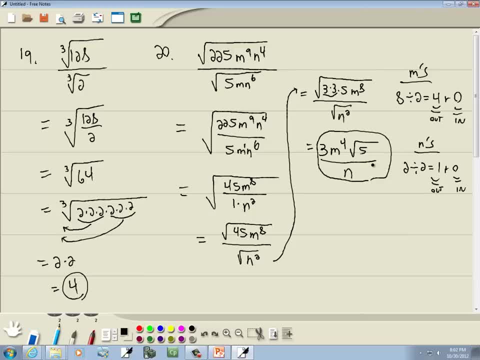 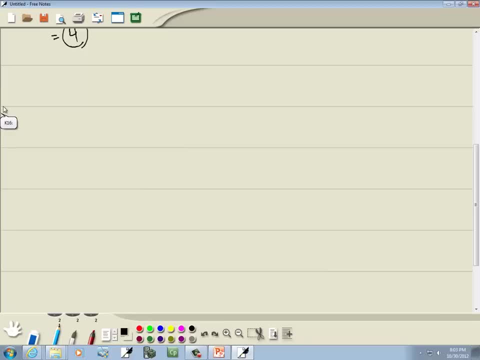 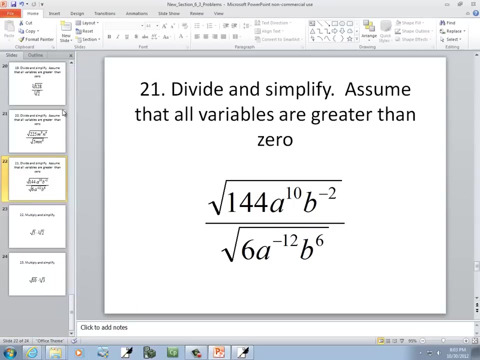 And that's our answer. Let's take a look at one more of those. So we've got square root of 144, a to the 10th, b to the negative, 2, over. square root of 6, a to the negative, 12, b to the 6.. 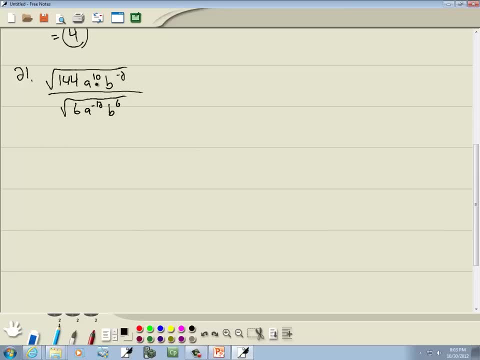 Now I notice that this has a, this has a, this has b, this has b. These look like maybe they would simplify a little bit- I'm not sure how much- So it looks like it would benefit us to put it into a single radical. 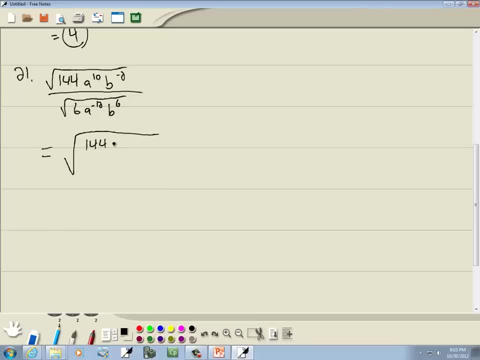 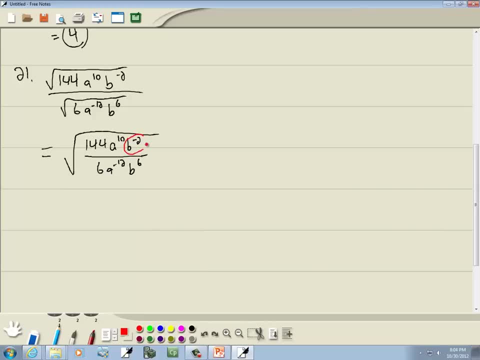 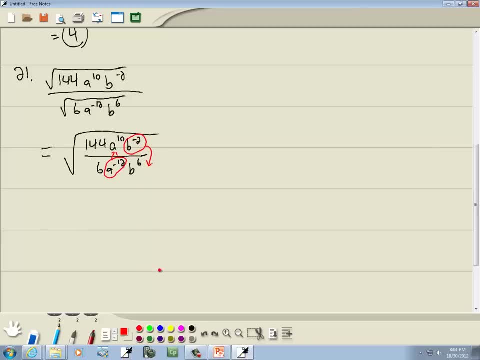 This a to the negative 12,. I want to take it up on top and it's going to become a to the positive 12.. Anytime you move anything opposite of where it's at in the fraction, the sign of the exponent changes. 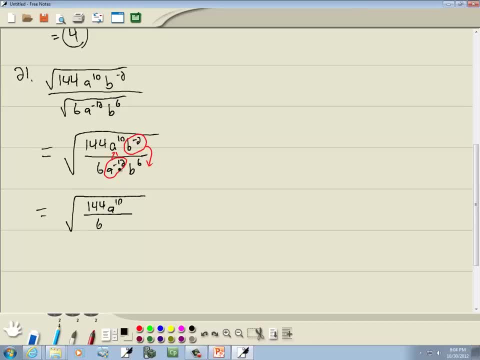 So I already have an a to the 10th up here. I move the a to the negative 12 up on top and it becomes a to the positive 12.. Now this one: I'm going to move it up on top and it becomes a to the positive 12.. 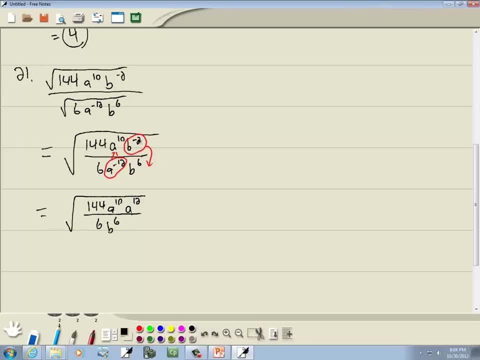 Now this one. I'm going to move it up on top and it becomes a to the negative 12.. So I already had a b to the 6. I take b to the negative 2 downstairs and it becomes b to the positive 2.. 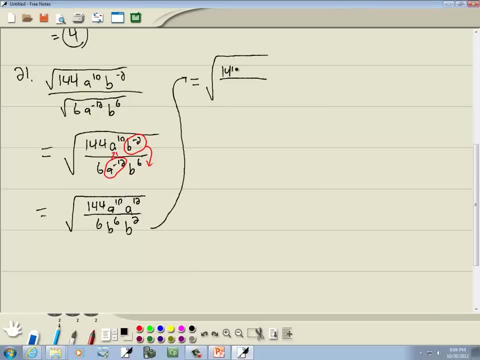 Now I can simplify those a little bit. a to the 10th times, a to the 12th is a to the 22nd, b to the 6 times b squared is b to the 8th. Well, the numbers. I can do something about this. 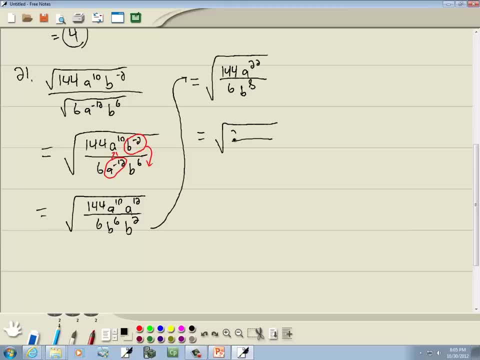 I can do something about this. Well, the numbers I can do something about this with six goes into that evenly, I think 24, 144 divided by 6 is 24, then a to the 22nd, B to the 8. okay, that's about as much simplifying as I can do with that. 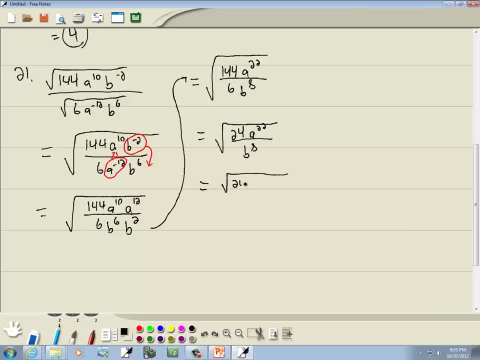 fraction, so let's split it back apart. we only put it in there temporarily so we can simplify a little bit. this right here definitely looks a lot easier than our initial problem. okay, 24, that's um 2 times 2, 2, 4, 8, 24 a to the 22nd and then. 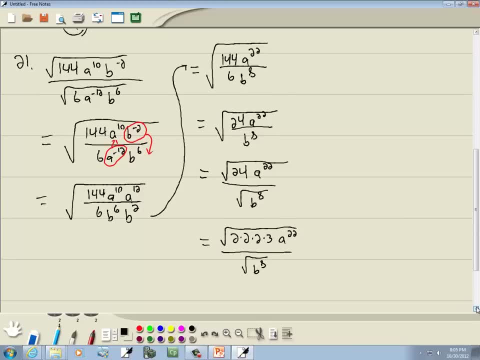 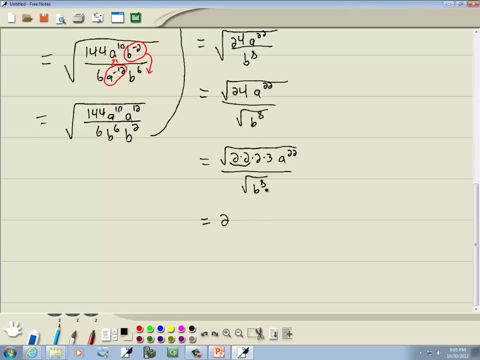 down here, B to the 8th, we're dealing with the square root. so, looking for a pair of something's, here's a pair of twos that's gonna come out in front as a single two. now for the A's. take our power, which is 22 divided by our index. this is a square. 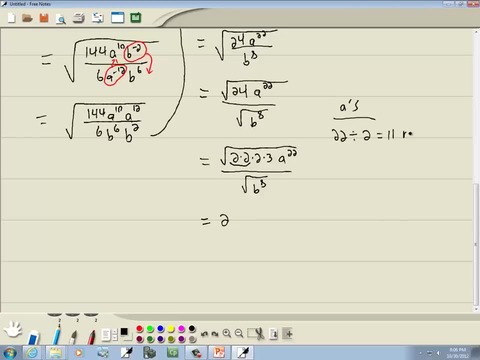 root, so it's by default 2. that gives us 11 or remainder of 0. so this is how many A's come out. we got 11 A's coming out and 0 A's staying in, so we're gonna have a to the 11th. the square root 2 times 3 is 6. that's staying inside down below. 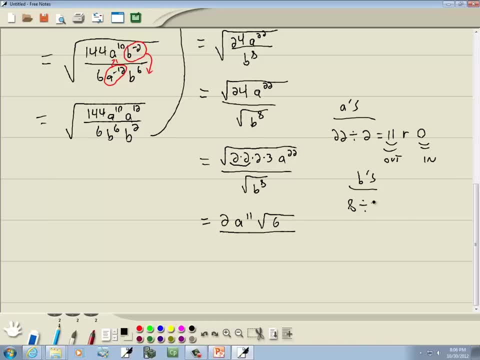 our B's, our power is 8 divide by our index, which is 2, it's a square root, so it gives us 4 with remainder of 0. so we're gonna have four B's come out and we'll have 0 stay in. so we've got B the fourth, and our radical disappears, since there's no. 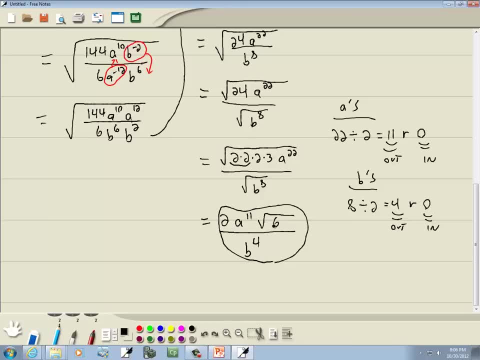 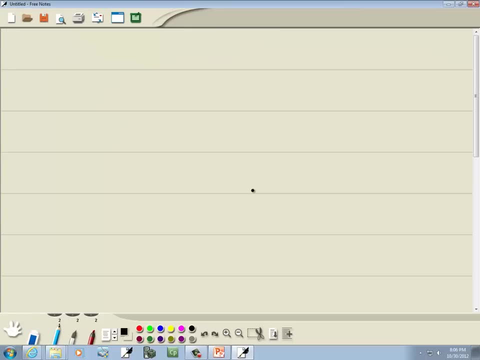 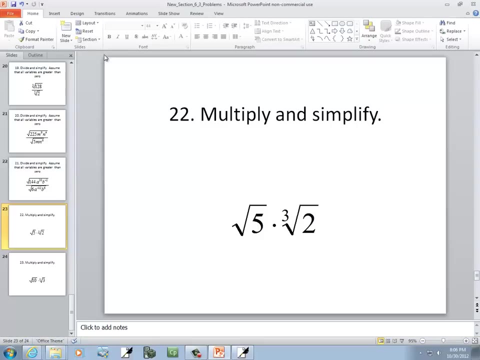 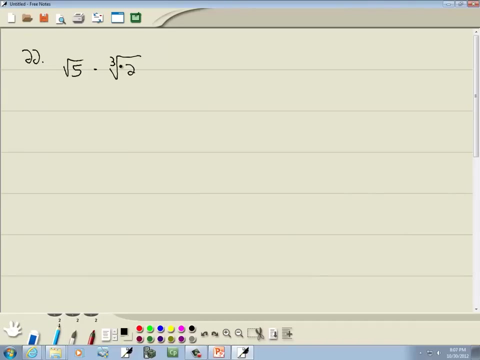 B's left inside, and that's your answer. let's look at these next problems. it's kind of a little bit weird. trying to really demonstrate when can you multiply radicals together is what you're trying to trying to emphasize here. Let me grab a drink. 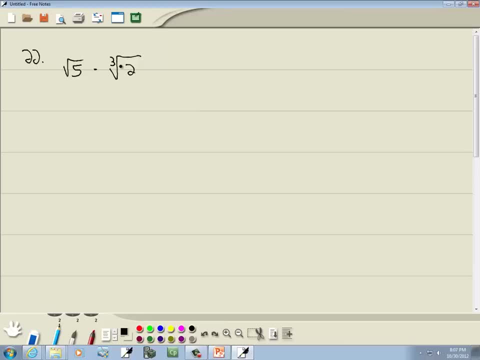 Okay, We can't multiply these radicals together. The indexes are different. Whenever the indexes are different, you can't, can't multiply them together. Well, let's write these in rational exponent form: fractional power. This becomes five to the one-half times, two to the one-third. 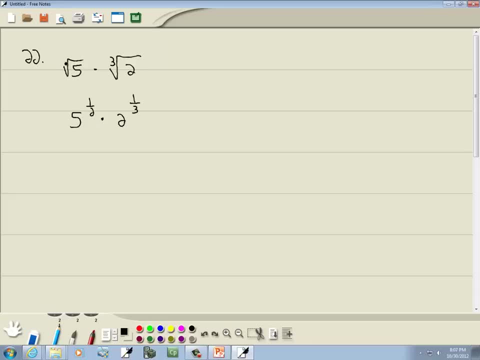 Whatever number is in this little slot right here that's called your index. Since there is no number here, it's by default two. it's a square root, so we put a two here and then we put a one up on top. Now in this one. 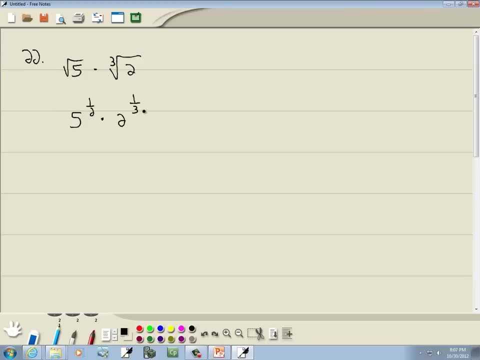 this was the cube root. so the number in the little slot here, our index is three. so that's why we put a three in the denominator and then it's by default one. Now think what I've just said. The index is what goes in your denominator. 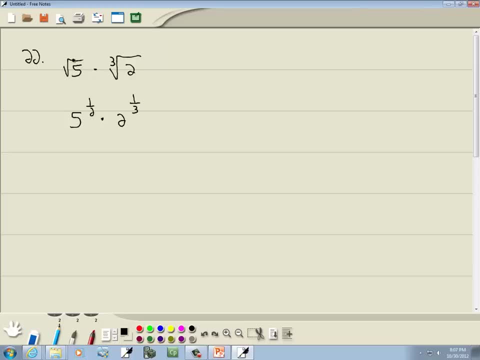 So the index is what goes in your denominator. If the index is the same, we could multiply these together, So all we have to do is get these indexes the same, So I need to rewrite them with the same number. This is two and this is three. 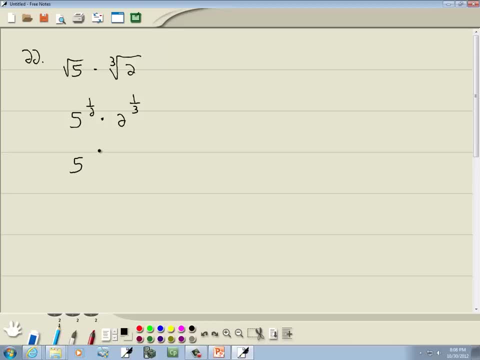 Basically, we want to get a common denominator, which would be six. Now here I multiply this bottom part by three. so we multiply the top part by three. So we got five to the three-sixth times. here I multiply the bottom part by two. so we multiply the top part by two. 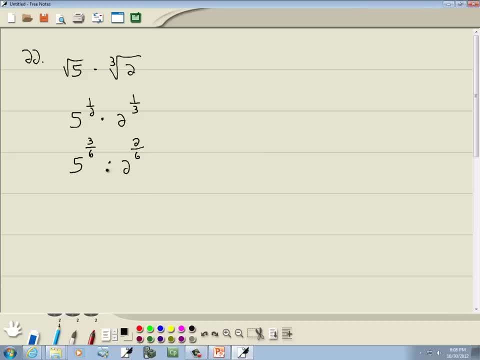 Like that. Well, now the denominators are the same and the denominator is your index. so we can put this back into radical form and the six would go here and then we'd have five to the third times. six goes here and then two squared Again. how it works is whatever is in your denominator. 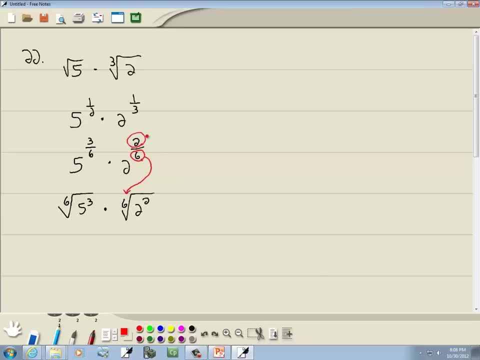 is your index. It goes in the slot there. Whatever numbers on top is your power that you can put inside. Well, now, these both have the same indexes, so we can multiply them together. So we got five to the third times two squared Um. 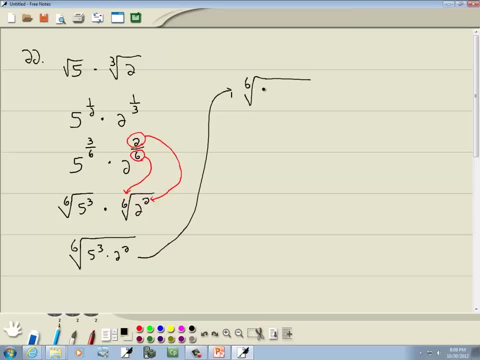 Five to the third. Five times five is twenty-five times another five is a hundred and twenty-five Two squared is four, So that gives us six, root of something. Two, eight, zero one, not not five hundred, Is that right? Two fifty, Yeah, five hundred. 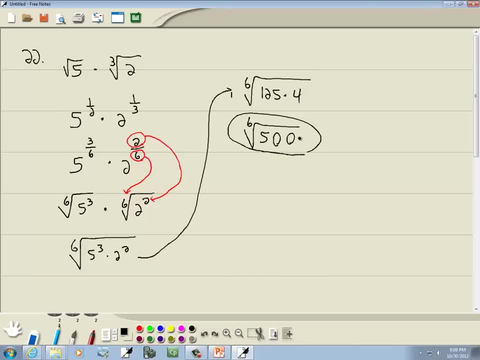 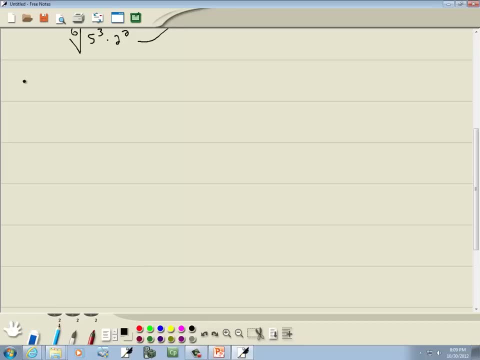 So that would be our answer. Let's look at this one. We've got square root of ten times a cube root of three. Now, this is a square root, so it's by default. our index is two. This is a cube root, so by default, our index is three. 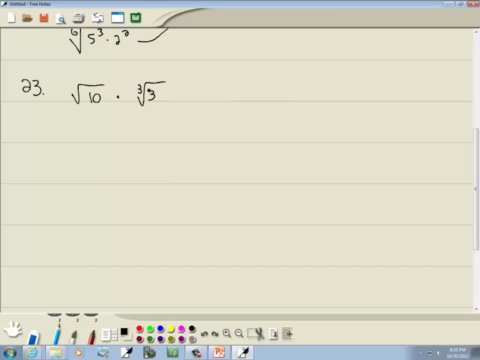 I can't multiply these together because the indexes are different. Well, we can put into rational exponent form, fractional power. So this one would be ten to the one-half times three to the one-third. Again the index. whatever numbers in the slot here goes in your 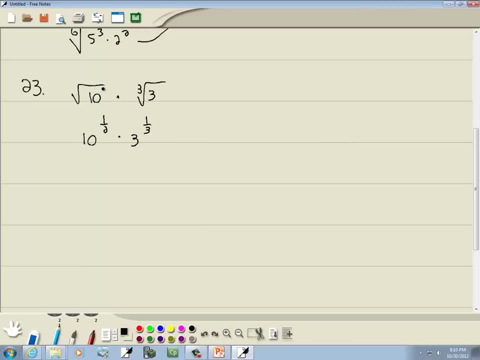 denominator. whatever power is here is by default one. if there is no power, goes up on top Here. the index is three, so it goes in our denominator. The power is one, so it goes up there Again. for us to multiply these together they have to have the 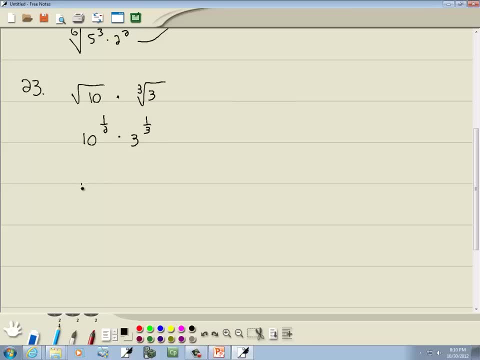 same indexes. So we have to get same denominator. So this one becomes ten to the three-six, and this one becomes three to the the two six. here I multiply top and bottom by three. here I multiply top and bottom by two. well, now they have the same denominator, so I'll put them back in the 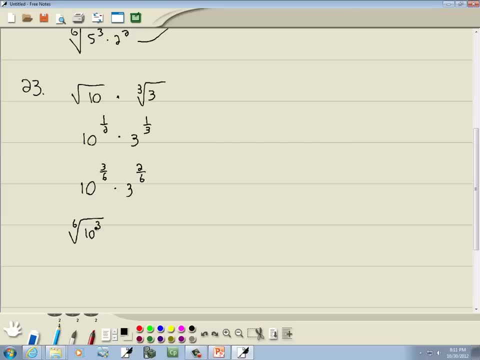 radical form. so this would be six and that'd be ten to the third, and this one would be six and this would be three squared. let's see what that gives us: six, ten to the third, times three squared. and I'm trying to think if this works out nice in any sense at all. I don't think it does. 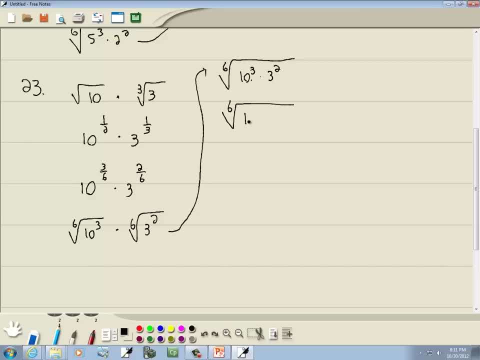 so ten to the third is a thousand. three squared is nine, so that gives us nine thousand. sometimes in these problems, after you merge them together like that, you may have something that looks like this: six here and then you have five to the third and two to the ninth, or something like that.